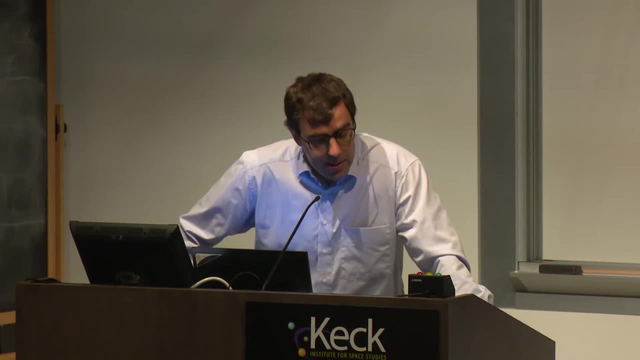 Dr Karl Stapelfeld. Karl is the chief scientist of the NASA Exoplanet Exploration Program at JPL. His research interests include protoplanetary disks and debris disks, high contrast imaging, exoplanets and star formation. So Karl earned his bachelor degree in mechanical and aerospace. 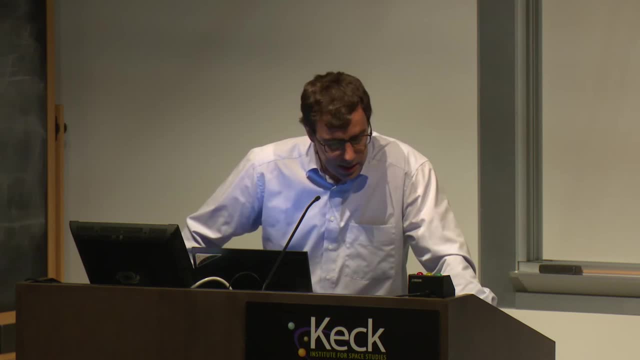 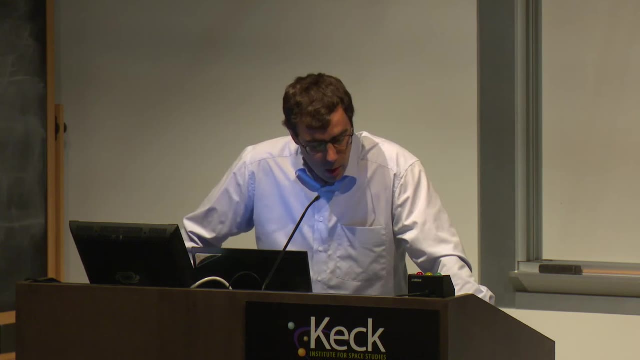 engineering and engineering physics from Princeton University and a PhD in astrophysics from Caltech, Karl started at JPL in 1993.. He worked on the Hubble Weave Peak 2 science and he was part of the science team. In 1999, he moved to the Spitzer Space Telescope Project Science Office. 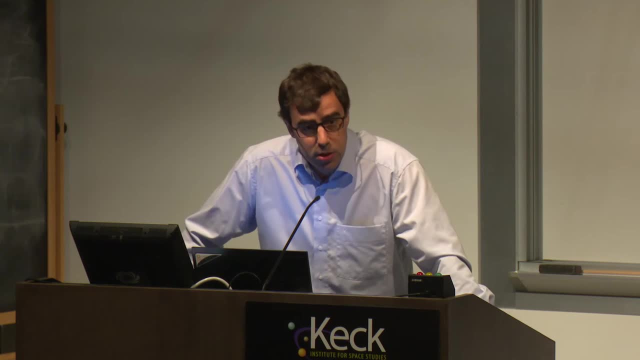 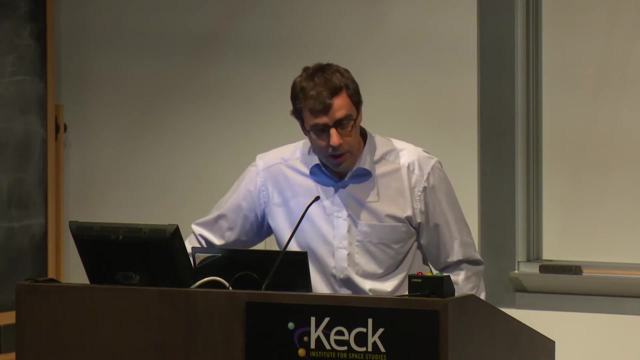 From 2002 to 2006,, he was the study scientist of the Terrestrial Telescope TPFC, And from 2011 to 2016, he moved to the NASA Goddard Space Flight Center, where he was the chief of their exoplanet. 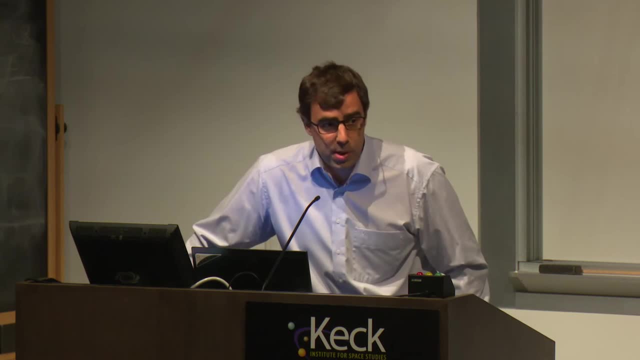 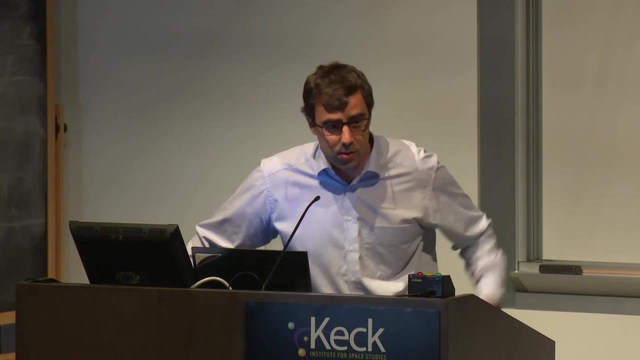 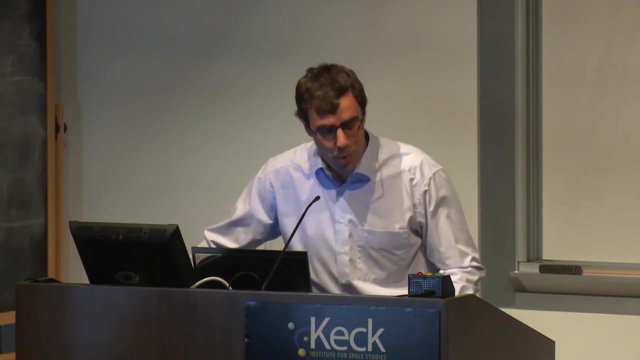 and stellar astrophysics laboratory. Karl returned to JPL earlier this year to take his position as the NASA Exoplanet Exploration Program chief scientist, And so, Karl, please. we are all looking forward to hearing about the overview of exoplanet direct imaging science from your point of view. 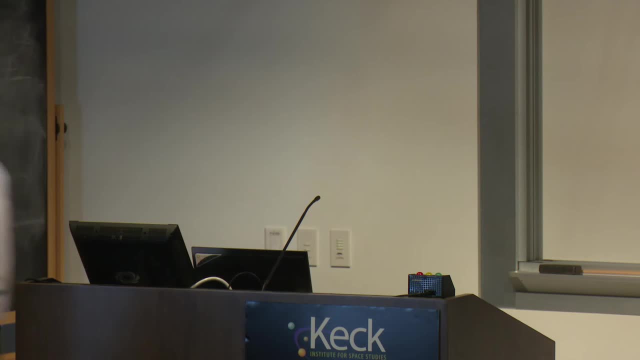 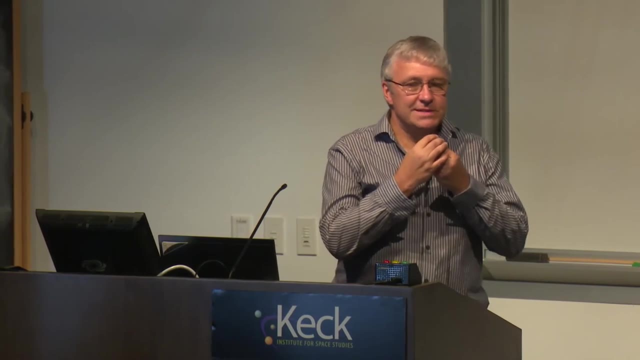 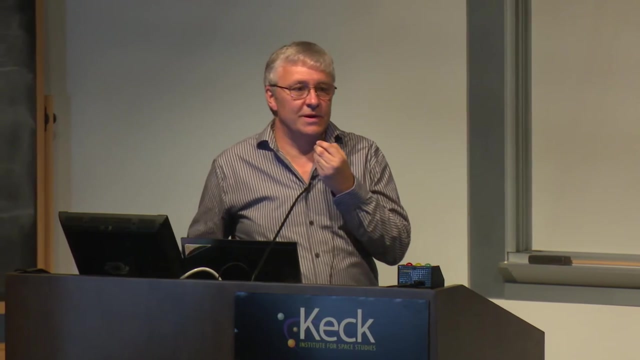 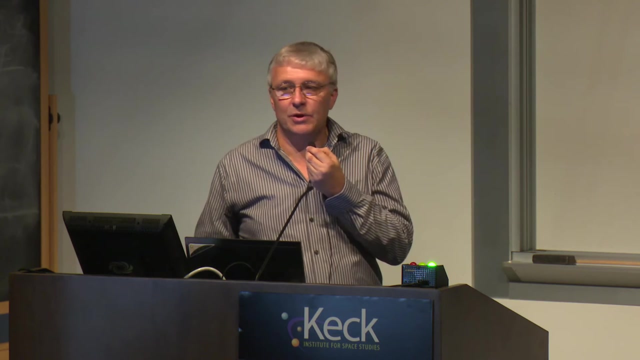 Thank you. Thank you, Dmitri. Well, I'm very glad to be here as a Caltech alum, as a returning JPL'er, and I really see this kind of event as something that's going to be beneficial broadly, including to the exoplanet exploration program as we develop, you know, new strategies for being better at high. 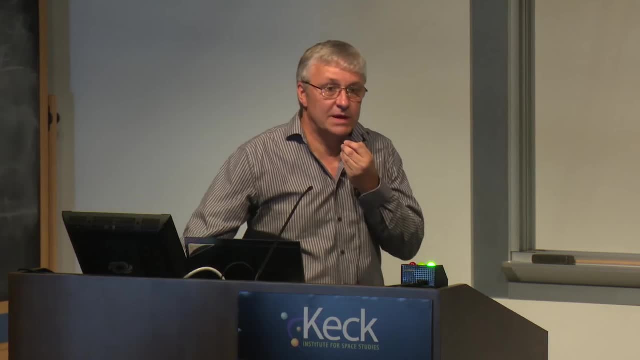 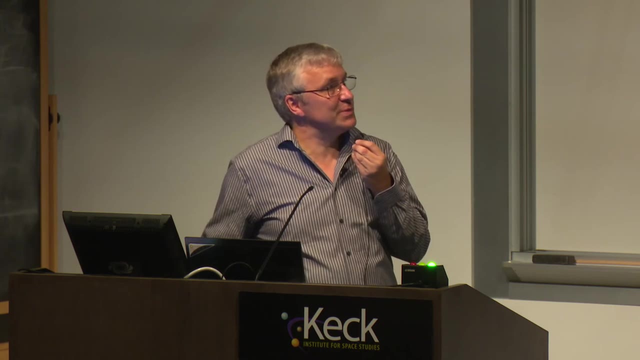 contrast imaging through the discussions this week and the other things that I hope come out of the meeting. So I'm enthusiastic for the week going to give you now an overview of exoplanet direct imaging science. I was asked to give it at the 101 level. I can see several people in the audience who 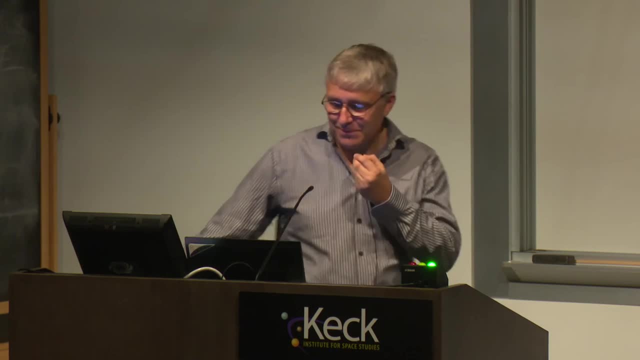 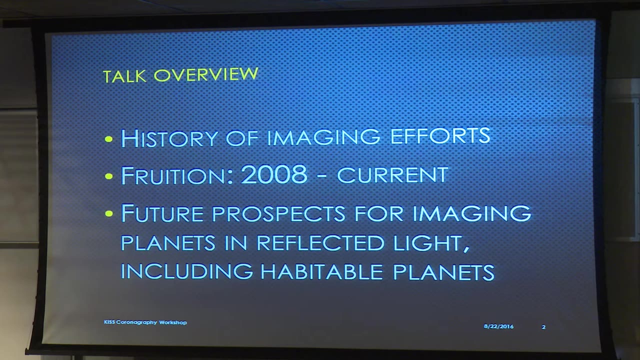 were at the 501 level, so you may not be too excited by what you're seeing, but we'll see how you take it, And so I think I'm just going to get started. So the way I'm going to approach this is to try to tell you my view of what was important. 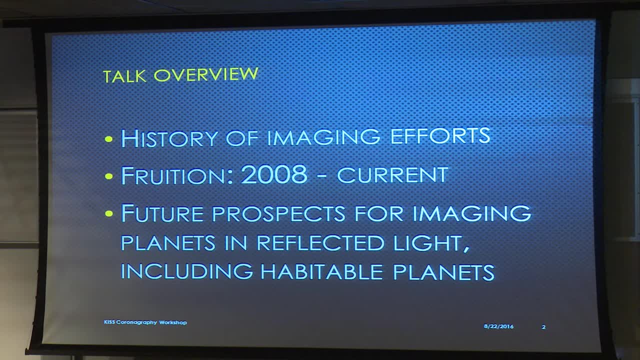 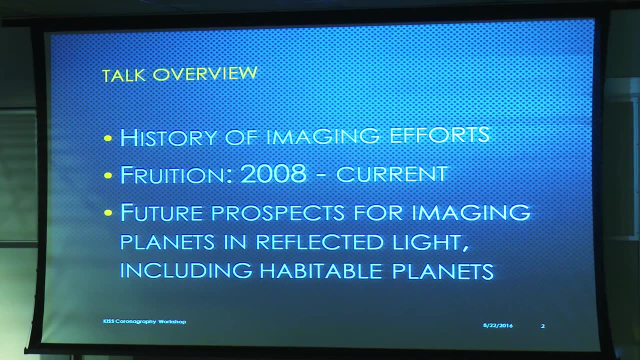 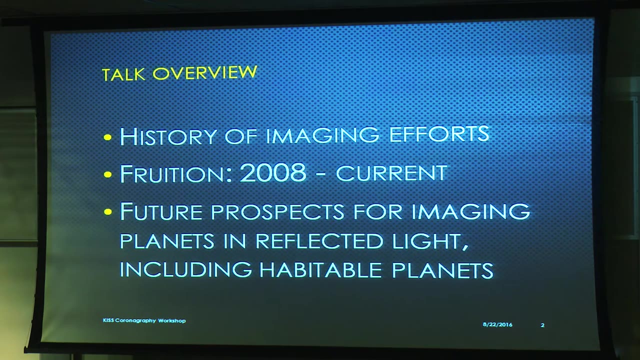 in history over the past 30 years or so in getting us to the point of having exoplanet images that we're enjoying today, especially the period starting in about 2008, where we really started to have the detections roll in, And then because the exoplanet program thinks ahead for NASA for large missions. I'm 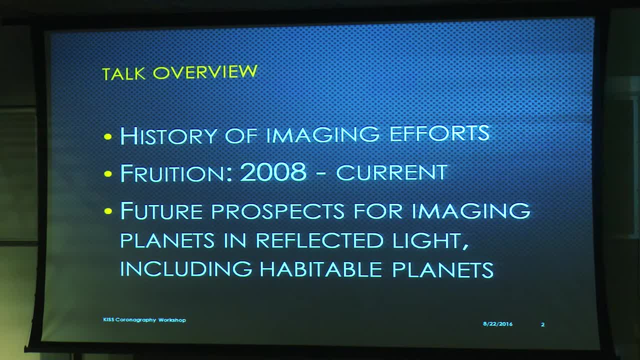 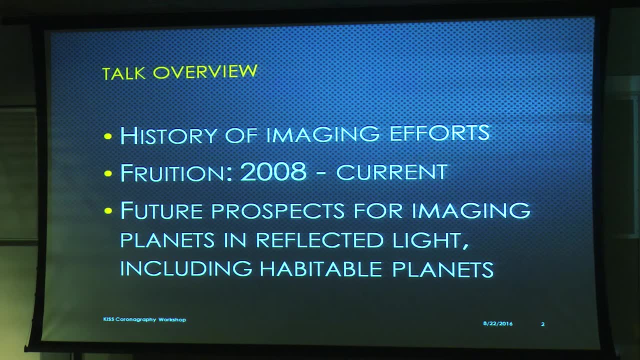 going to talk to you a good bit about the requirements for imaging planets and reflected light, including that crucial problem of habitable planets that the 2010 decadal survey thought was a priority for future investments and hopefully will be something that the 2020 decadal survey decides not to do. 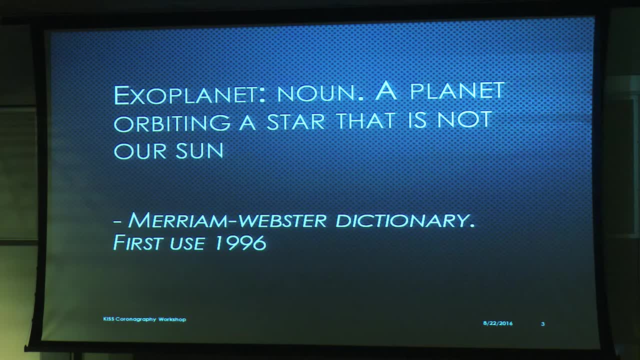 Thank you. So let's start out on what's an exoplanet. It's more basic than that: A planet orbiting a star that is not our sun, according to the Merriam-Webster Dictionary, And according to them it's also first used in the year 1996, so it 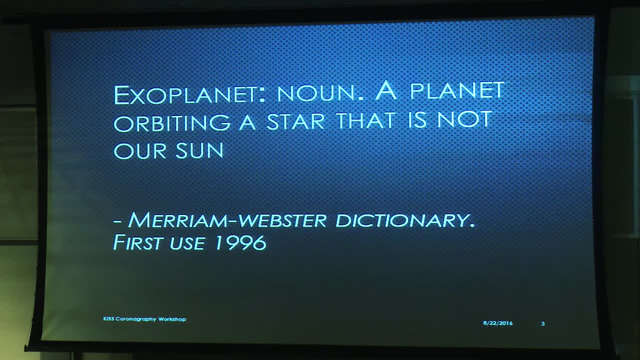 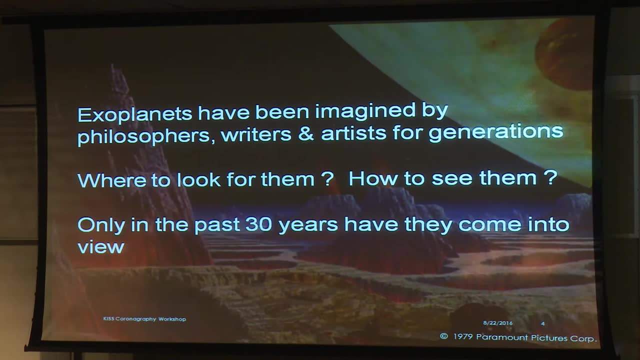 is definitely a recent term, even through years of science fiction and philosophy and so forth. I don't know that anybody was using this term earlier than 1996.. And of course there was a lot of imagination about what exoplanets would be. 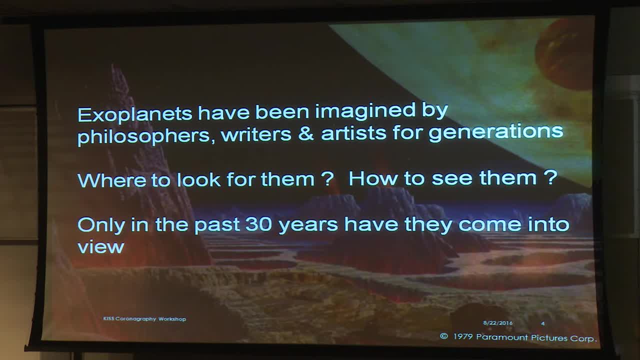 how many would be out there? lava planets, ice planets, planets that are all oceans in a bad Kevin Costner movie. So we've had lots of imagination, but science is in a position to look for them in many different ways, And so now, as I said, 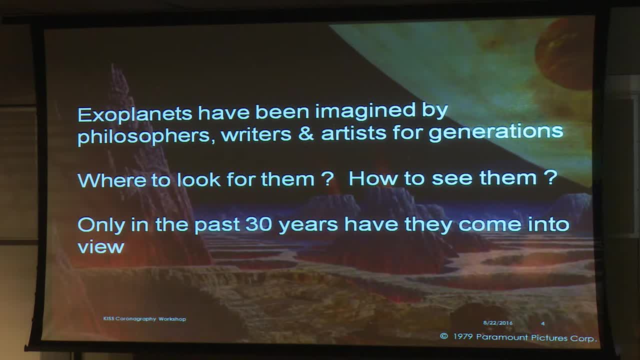 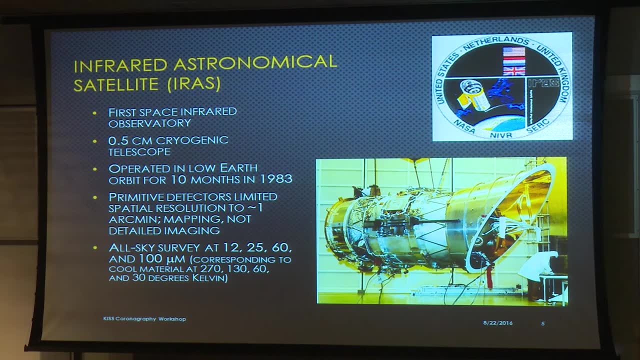 earlier. they have come into view during the past 30 years. So that was a process that, in my view anyway, started here with a project that JPL was doing and that led to the creation of the Infrared Processing and Analysis Center, which is a 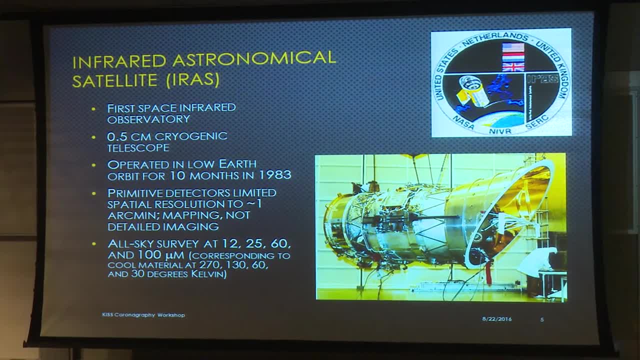 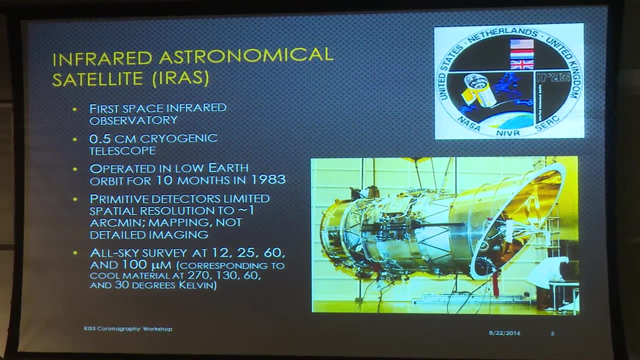 and that is the IRAS all-sky survey in mid-infrared and far-infrared wavelengths. that took place back in 1983.. Now you're going to see a continuing theme here, that we are doing things on exoplanets with a general-purpose telescope. 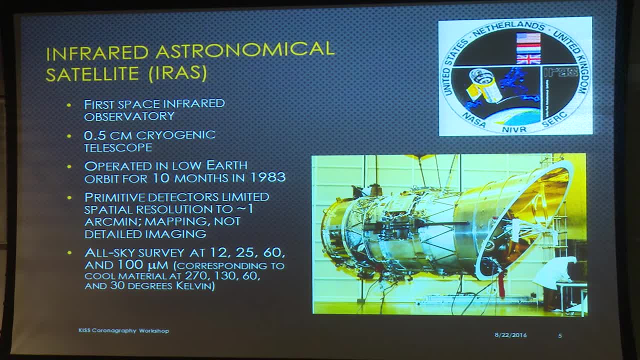 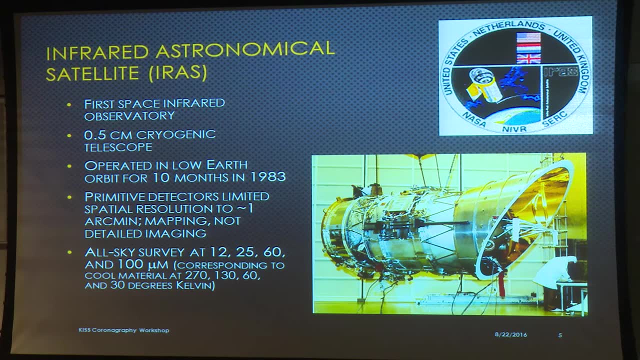 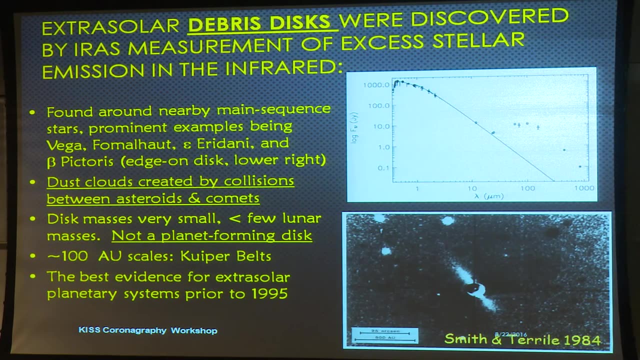 that really wasn't designed specifically for the exoplanet application, but nevertheless it does lead to important insights. It was an all-sky survey, not really targeting any one particular object at a time, and it had four bands and the main discovery relevant to exoplanets of the mission. 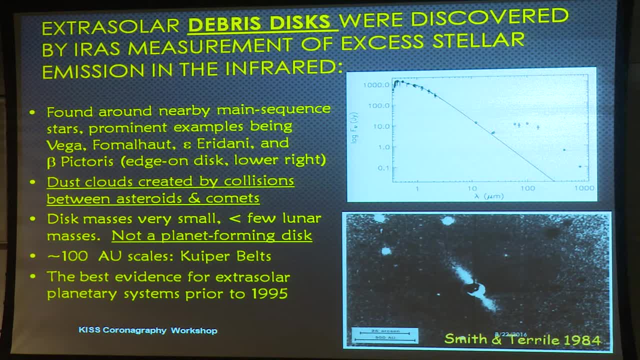 was that there were stars out there that had infrared signals well in excess of what they should have been if there was a bare stellar photosphere alone, especially out here, starting at 70 and 100 microns. There were lots of stars earlier type, higher luminosity stars that showed this excess. 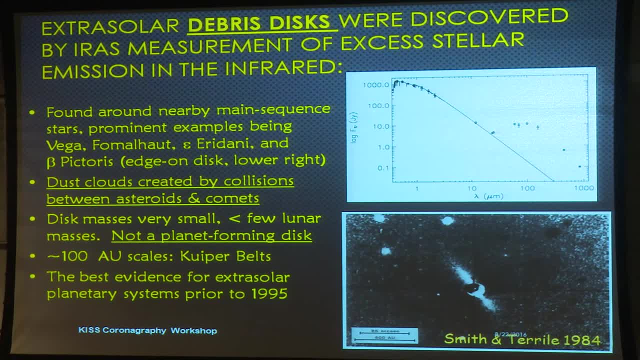 There was, of course, the state where Vega was above, which was observed early on in the calibration target, and it proved to not be a good calibrator at all because of this excess. So nearby stars were prominent, having this infrared excess. 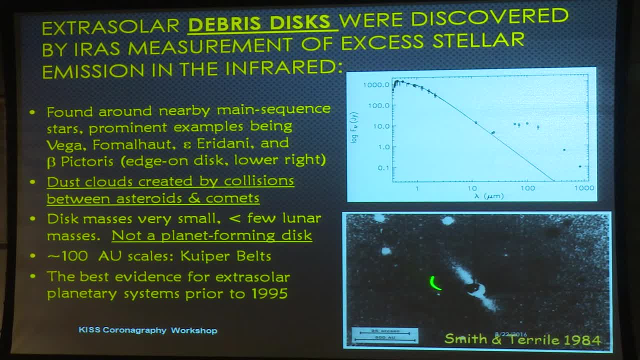 and Brad Smith and Rich Terrell went to the telescope in Chile in 1984. They were interested in moons around planets so they had a coronagraph. They put it at several of these stars and Beta Pictoris turned out to have this disk-like cloud seen nearly edge-on. and they were interested in moons around planets and they had a coronagraph. They put it at several of these stars and Beta Pictoris turned out to have this disk-like cloud seen nearly edge-on. and they had a coronagraph. They put it at several of these stars and Beta Pictoris turned out to have this disk-like cloud seen nearly edge-on. 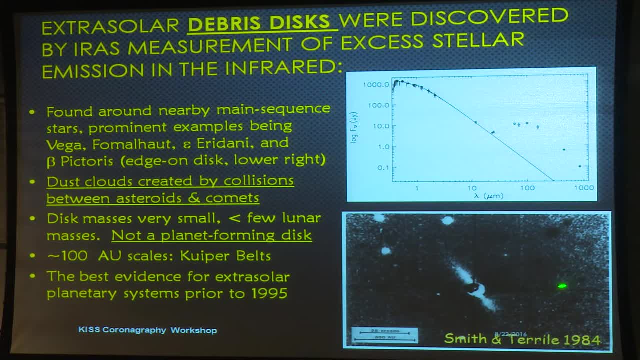 and this is basically the first direct imaging evidence of another planetary system. and this is basically the first direct imaging evidence of another planetary system. Later work found that these dust clouds had to be created by collisions between parent bodies and constantly replenished because the small particles in the disks would blow away, given enough time, over tens of thousands of years. 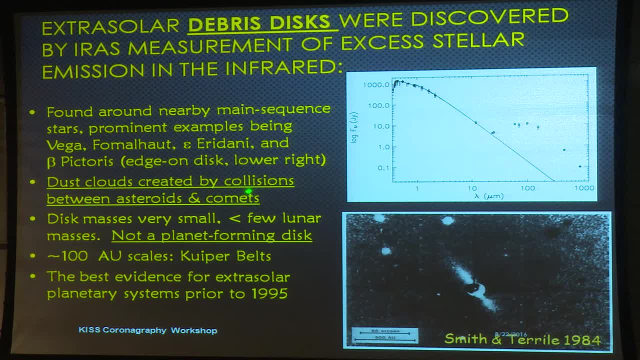 and so they required parent body belts, like our asteroid belt or like our Kuiper belt, in order for this structure to persist. The mass of material in these disks is very small, less than a few lunar masses, so this is not a stage of planet formation, except perhaps of large rocky planets. 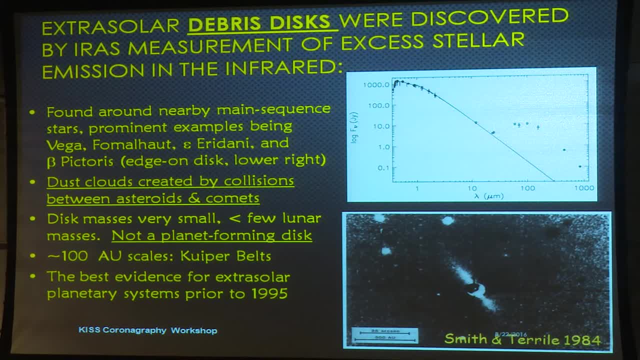 The gas is basically gone. so if there are Jovian planets- and we know there is one- they've already formed. And, of course, this was the discovery of a Kuiper belt around another star, before we even knew that our own solar system had a Kuiper belt. 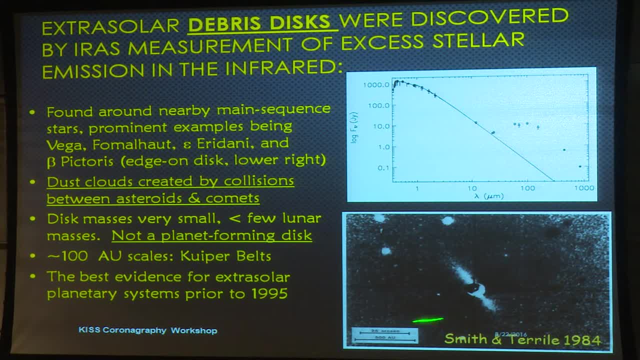 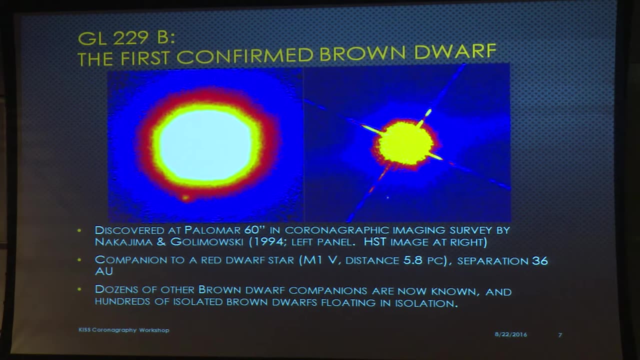 That didn't come until 1992, and if you were in grad school, like myself in the early 90s and late 80s, and you wanted to work on extrasolar planets, this was the biggest thing going. So from looking for disks around stars with infrared excess, 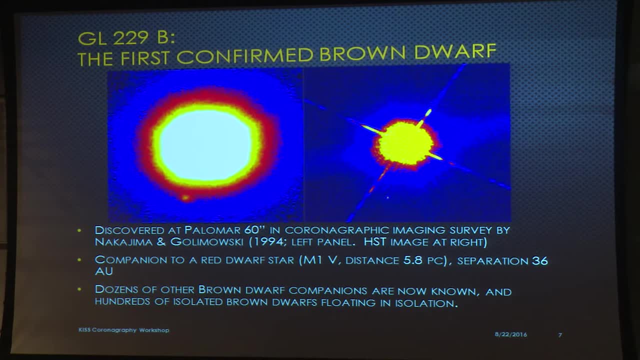 there were long predicted to be brown dwarf objects that would be stellar, substellar objects that were not massive enough to sustain nuclear fusion in their cores, And people would look for these faint objects near M stars, late-type stars of low luminosity, because they would be the easiest contrast challenge. 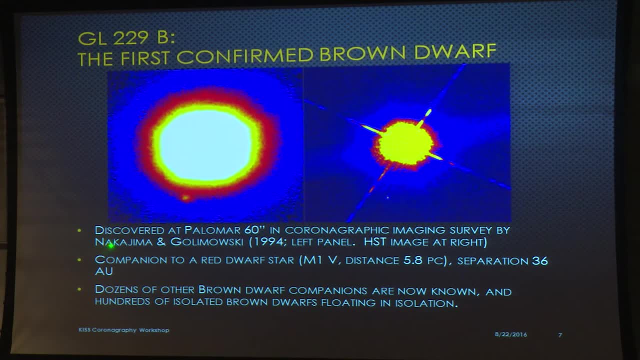 So this is the discovery of a Kuiper belt, Every image that Tadashi Nakajima and David Golomowski obtained, also here, involving Caltech at the Palomar 60 inch. they didn't have a really good adaptive optic system, it was just seeing limited. the companion was just barely seen over there. 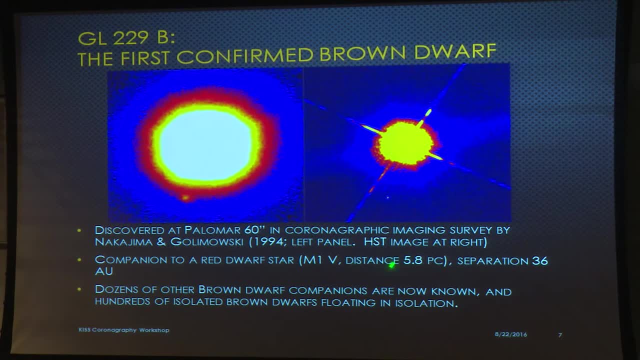 You could see a little bit better in the Hubble Space Telescope And this is a nearby star at 6 parsecs, a 36 AU separation companion, And this sort of kicked off the search for companions in a big way after this discovery. 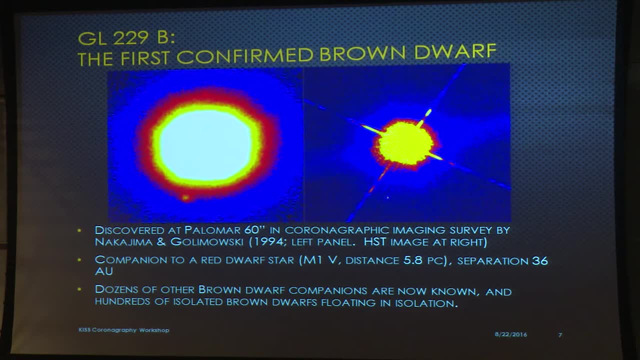 Today there are dozens of brown dwarf companions that are known from surveying a lot of objects and there are hundreds of field brown dwarfs that were found from the 2MASS survey, from the Sloan Digital Sky Survey, And the distinguishing feature of these objects that links them to planets is the spectrum. 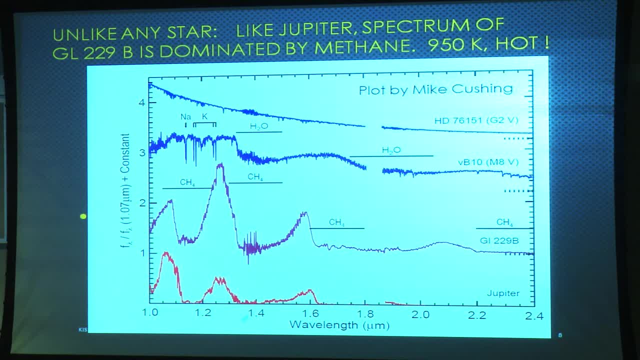 So we're showing here four different spectra of the Sun, here at the top, going across the near-infrared wave bands. Then here is a late-type M star near the end of what we thought was the star. This is a stellar sequence at the pre-2MASS era. 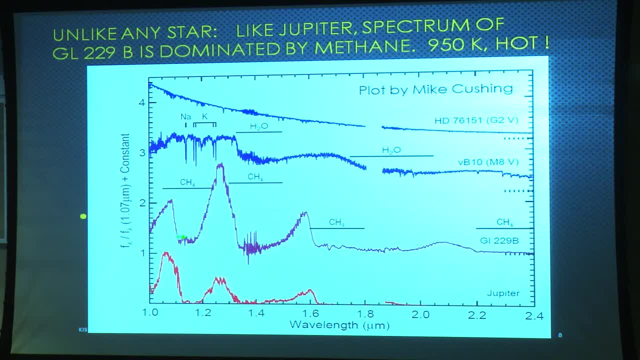 Here's the spectrum of GL229b, the brown dwarf companion that I just showed you, And here's the spectrum of Jupiter at the bottom, And, of course, the thing to notice is that there's a huge similarity between Jupiter's spectrum and the brown dwarf spectrum. 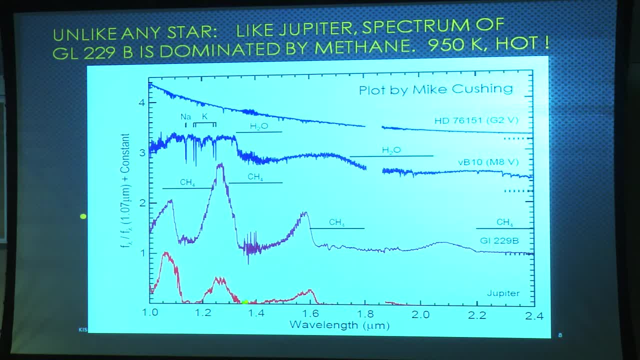 Nothing at all like even a late-type star or, of course, the Sun, And the key distinguishing feature is the presence of methane. Jupiter is a 120 Kelvin effective temperature. object GL229b is more like 900 Kelvin, But nevertheless they share these deep absorptions from methane, and especially here at the 1.6 micron cutoff. 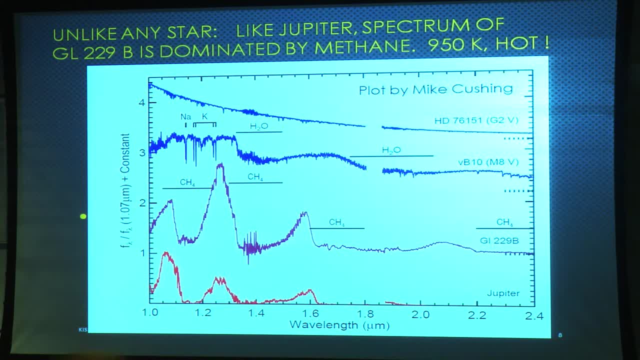 So there was nothing else in the sky that had methane in it other than our giant planets until this discovery took place, And that kicked off a lot of interest in doing surveys for companions that were methane-dominated like this, And that went forward through the 1990s and into the early 2000s. 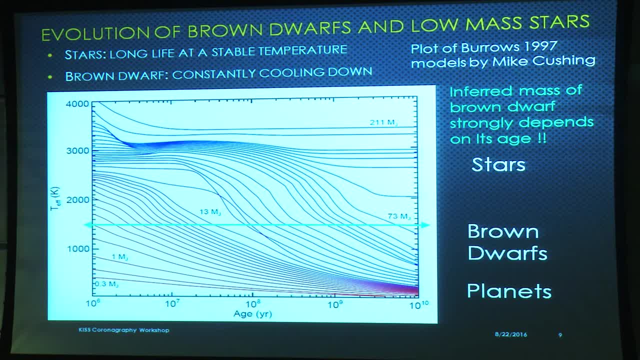 So an important feature of the brown dwarfs is their luminosity evolution. This is a set of tracks from Adam Burroughs 1997.. It shows the effective temperature of a brown dwarf as a function of its age, And so it is born with a lot of heat, of formation, gravitational contraction. 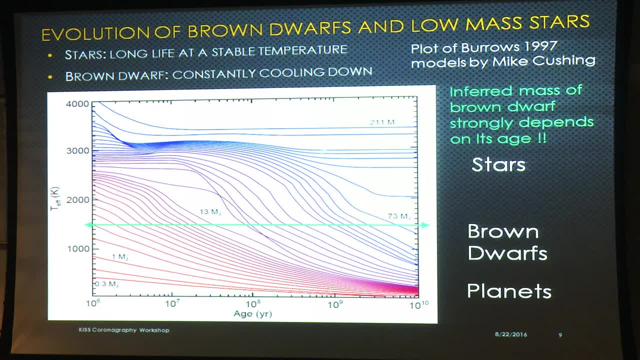 And if it's massive enough- 211 Jupiter masses is roughly 0.2 solar masses- then it comes down to the main sequence, to an equilibrium luminosity over here equilibrium temperature. But if the mass is not sufficiently large, then the luminosity plateau never happens and it just continues to cool down into oblivion. 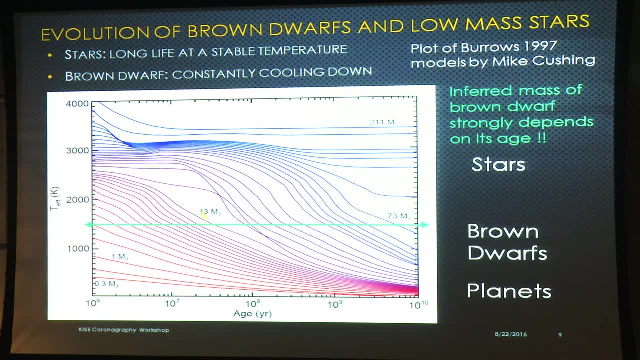 And then there's a special extra feature that happens at 13 Jupiter masses or so, where, above this, there is a little bit of a plateau caused by the burning of deuterium, a residual form of hydrogen that came in with the planet-forming gas. 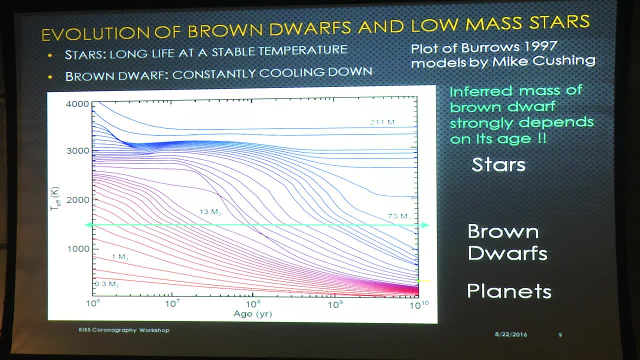 But then, after the deuterium is used up, it then still decays down away into cold and oblivion. And notice that each one of these curves is for a different mass of planet. So this is showing that a brown dwarf will cool, a planet will cool. 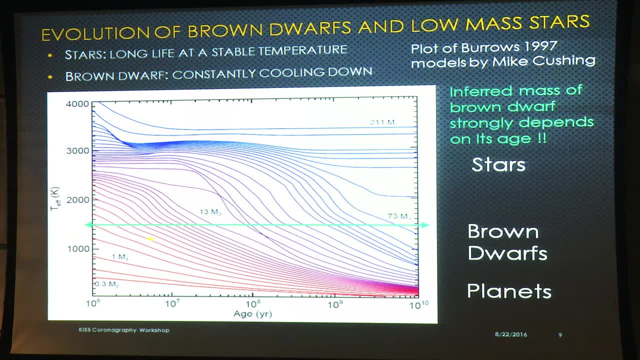 And let's say you find an object that's 1500 degrees Kelvin would be across on this line. So you've got to know how old it is in order to interpret what its mass would be. So if it's very young, it might just be a few Jupiter masses on this side of the diagram. 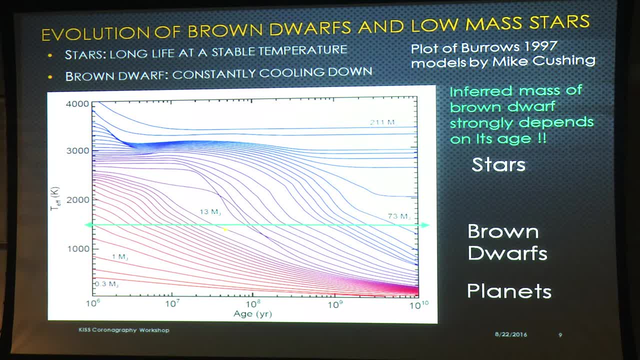 But if it's older, it could be above this limit of deuterium burning, Which is considered to be the boundary between planets and brown dwarfs, And so it could be out here being masses of, you know, 20 or 30 Jupiter masses. 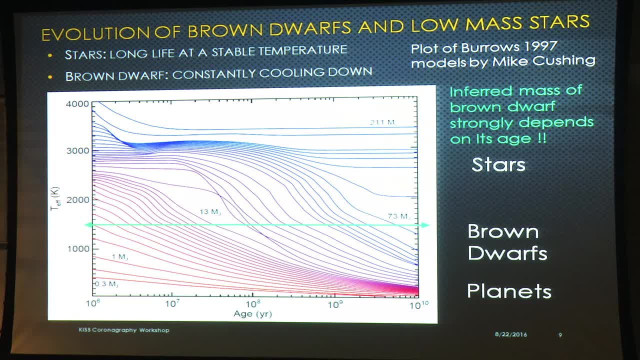 And if you go out this far it could be all the way up nearly to the hydrogen burning limit. So this put a premium on two things. One is, we really want to know the ages of the stars that host brown dwarfs. 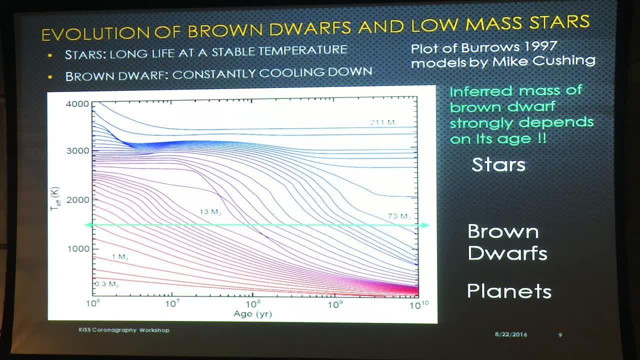 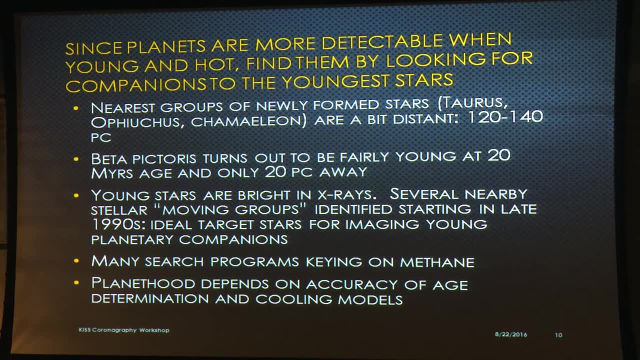 And second, if you want to find more of these methanated companions, the way to do it is to find samples of young stars and look very hard at those for companions in direct imaging. So the samples that you would look at are the most recently formed stars. 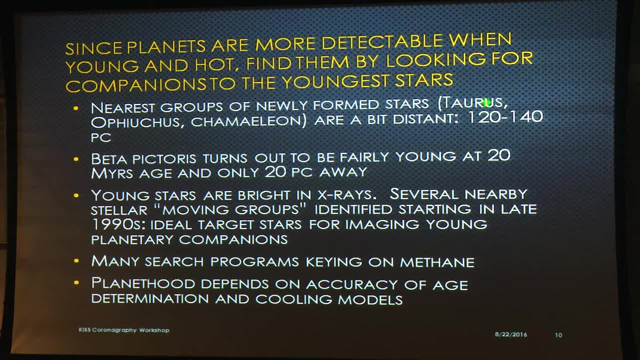 These are T Tari stars in constellations like Taurus, Ophiuchus and Chameleon, But those happen to be 120 parsecs away, So they're not easy to resolve and look in close. But Beta Pictoris, that original discovery image that I showed you from 1984,. 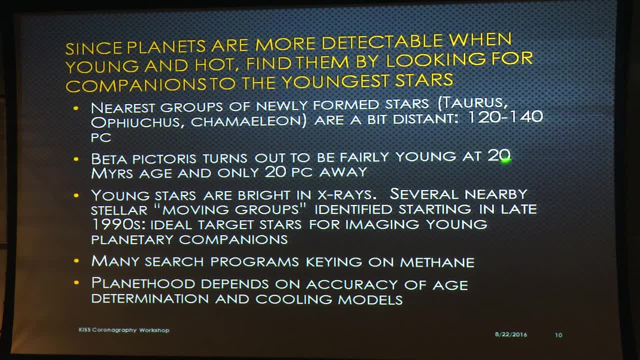 that turns out, after years of work, to be only 20 million years old and much closer, 20 parsecs away. So it was gradually realized in the late 1990s after the ROSAT satellite surveyed the sky in X-rays. 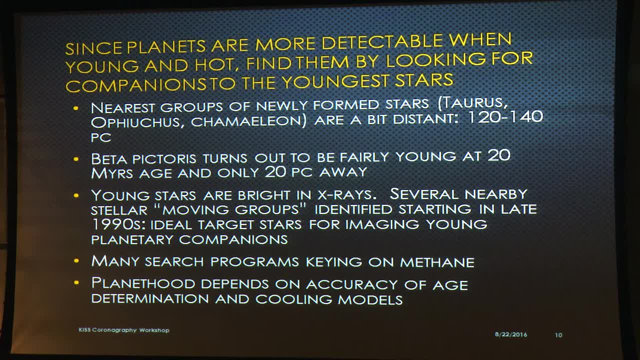 we were able to see where the chromospherically active stars were And we noticed- many workers noticed- that these stars were part of moving groups. They had common, proper motions and space velocities indicating that they formed in a young cluster, but a very loose cluster that was in the process. 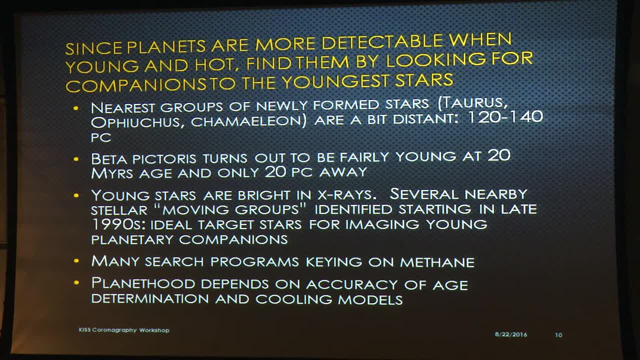 So they had a process of dissipating and distributing into the galactic disk And so you can catch some of these, these moving groups, and then make imaging searches for companions. And we're still doing that today. every time we get another improvement in contrast capability. 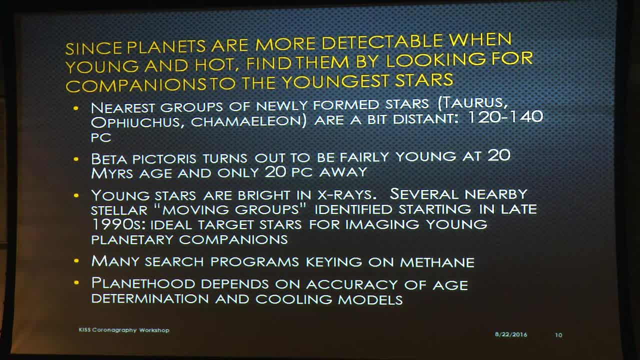 In the early days, these search programs were keying on methane, because that's what we saw in GL229B. It's later proven that that wasn't such a great strategy, as you'll see. And then, whenever a target is found, 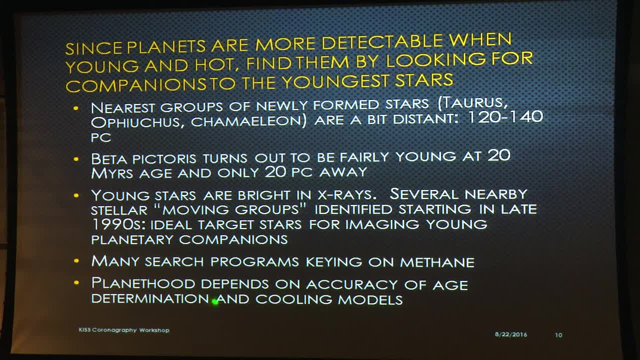 a companion is found, there's always a debate about whether it's a planet or a brown dwarf, because the age isn't exactly known And so it also depends on the cooling models. So you can't feel satisfied, as a dynamicist, that you know the mass of these planets. 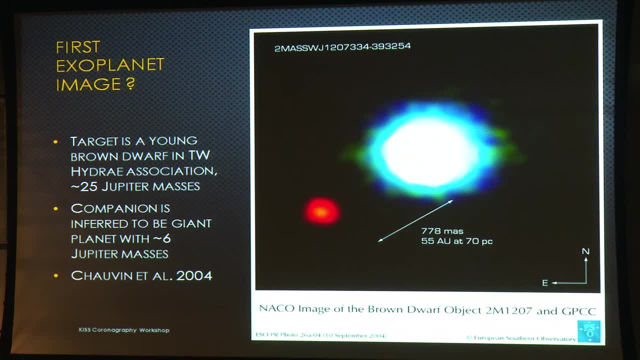 when they're actually detected. It's always going to be subject to revision, So possibly this would be the first image of an exoplanet made with the VLT in the near-infrared. It's in a star in a moving group. 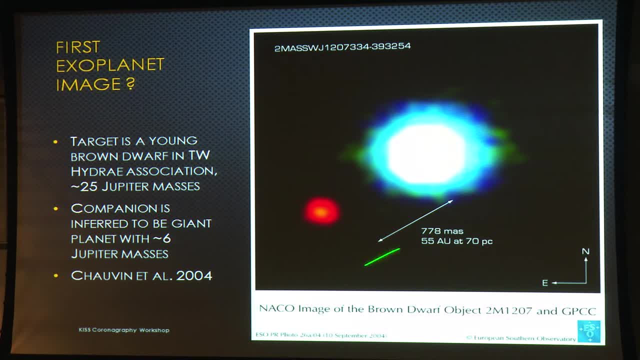 In this case the TW Hydra Association, And it's around a brown dwarf. The primary object is itself a brown dwarf And the companion object, 55 AU away, is substantially fainter The companionship, as always in these cases, 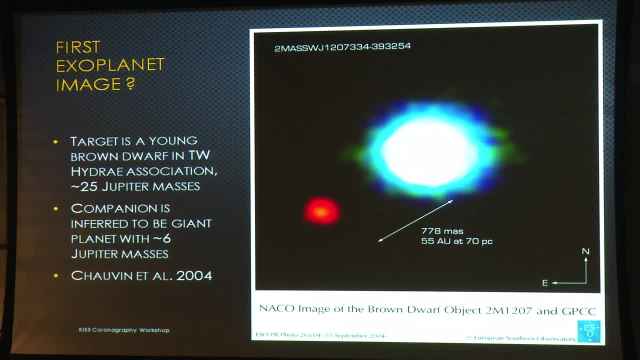 is verified by measuring the image separation multiple times and seeing that the companion shares the proper motion of its host star. And here the companion from the evolutionary track models comes out to six Jupiter masses. So this pretty much makes the case for being an exoplanet. 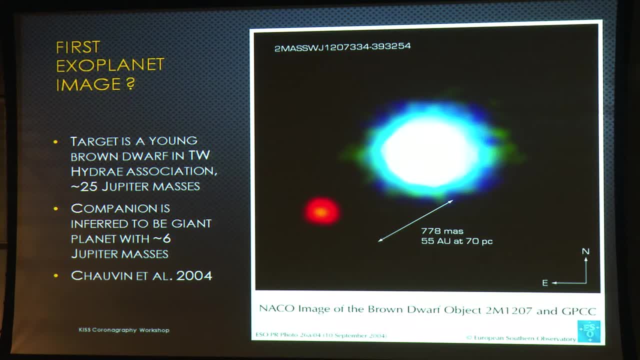 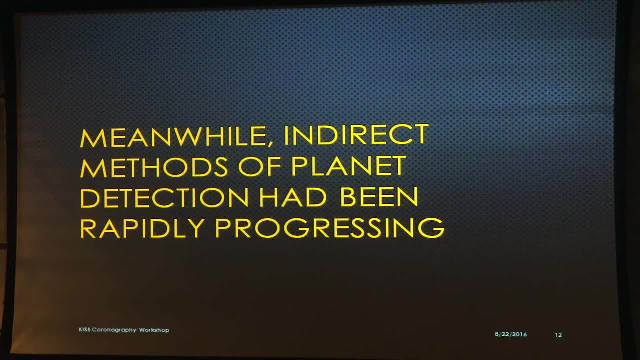 but it's not around a regular main sequence star. So if that's what you want for it to be a real planet, this is a halfway So. imaging is finding these companions around young moving group stars, especially ones that are dusty and young. 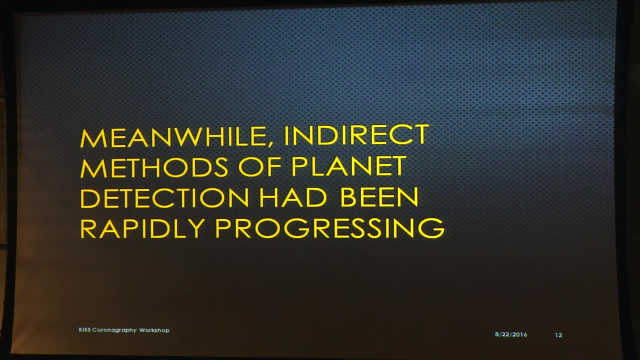 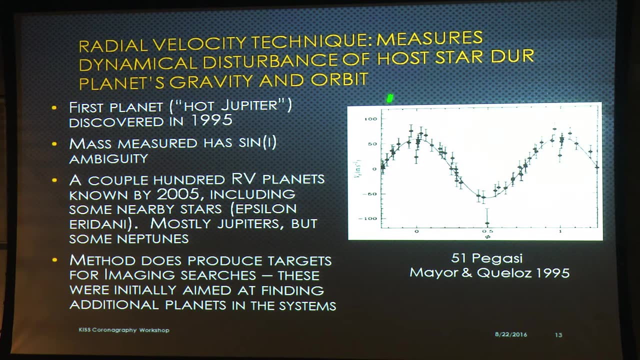 But at the same time as imaging is making progress here, there are other methods of planet detection. Now I'm just going to remind you of- and this is of course completely known to many of you. So the radio velocity technique measures the disturbance of the host star. 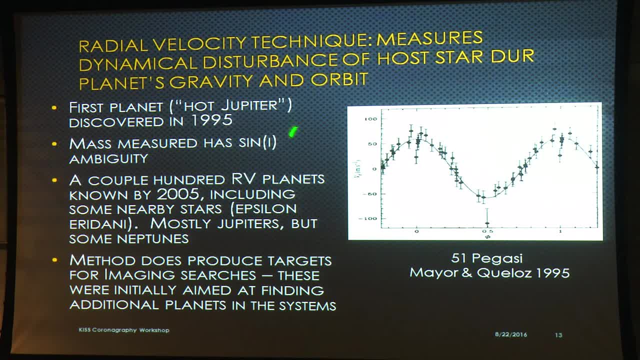 due to the gravity of the planet as it moves around its orbit. And so 51 Pegasus, just as you know from the 20th anniversary last year, was the first one of these found around a sun-like star in 1995.. 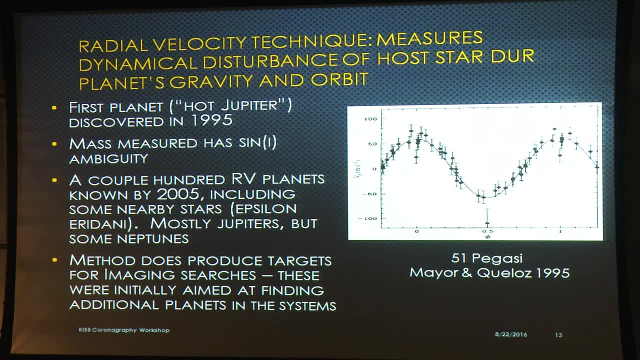 This was a very large amplitude, very close in hot Jupiter surprised the heck out of everybody. We would later be surprised in imaging about things that were in a parameter space. we hadn't expected either. As always in radio velocity you can only see the projected component of the velocity along the line of sight. 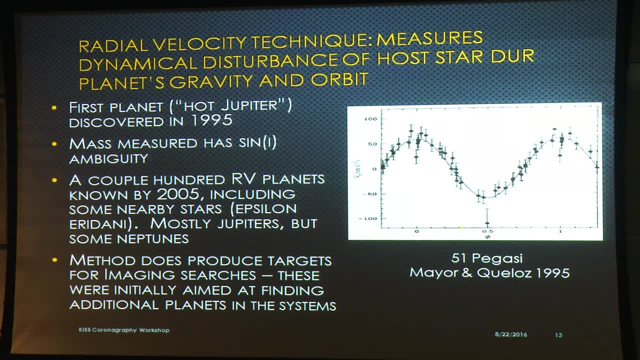 So there's always a sign-eye ambiguity. The mass you get is sort of a lower limit And by the time we got to 2005,, a couple hundred of these things were known, And this was especially interesting because some of them were around nearby stars. 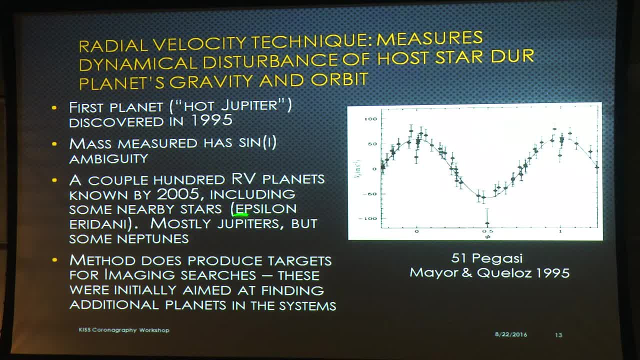 that were young and accessible to imaging. So I can recall, you know, trying to see the Epsilon Eridani planet at Palomar. I bet you many of you can recall trying to see the Epsilon Eridani planet at Earth. 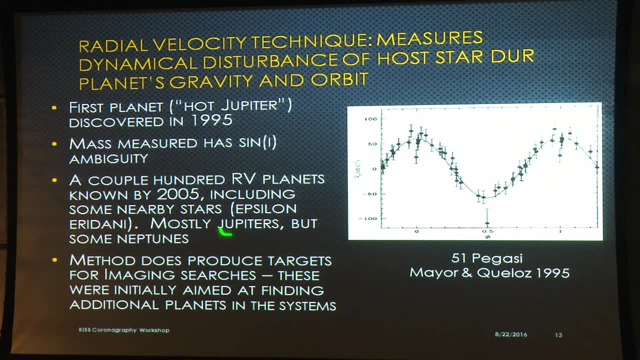 You can see it around some instrument that you were using. And these RV planets tend to be Jupiters, mostly in terms of their mass determination, subject to the ambiguity, And some of them are Neptune mass planets. So the good thing about radio velocity for imaging. 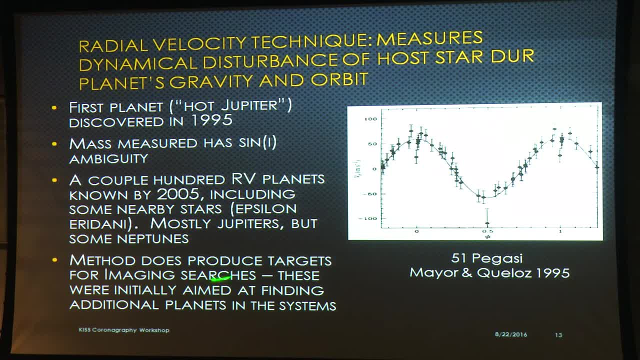 which is our purpose here, is that it does produce targets that imaging searches can go and follow up. And so originally, of course, these things are pretty faint. So when you go and look at a radio velocity planet system, it's because you're interested in seeing another planet that may be more massive. 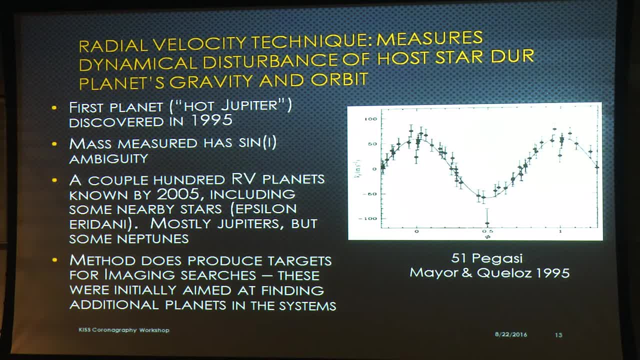 that hasn't shown up yet in the RV signal, And so some folks, like Justin here, have spent a lot of time looking for planets that are producing radio velocity trends- And of course they turn out to be stars sometimes- But we can thank the radio velocity folks for giving us a target list. 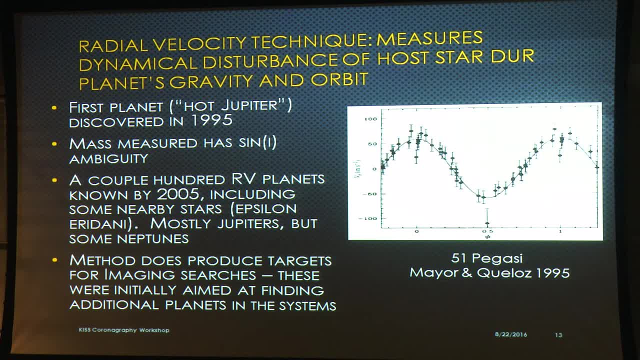 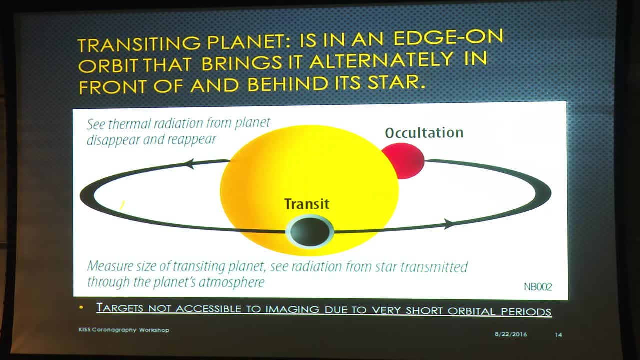 to aspire to in our future space missions. So transit Very basic here. as you know, When the planet is able to be in orbit, is able to be aligned with the star in almost equatorial orbit. it passes in front of the star and it disappears behind the star. 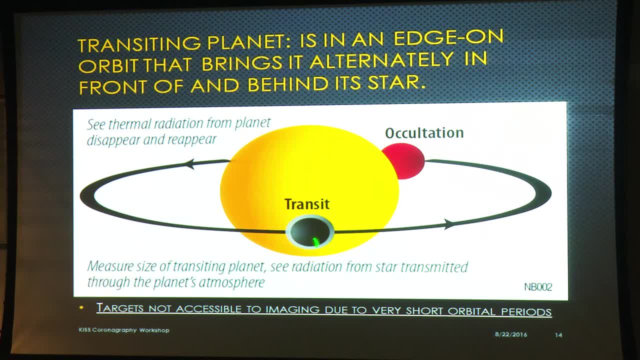 And you can measure the size of the planet from the size of the drops in the brightness of each as they go around. You can actually measure the temperature if it's hot enough to go into occultation. While this is a fantastic and productive technique, 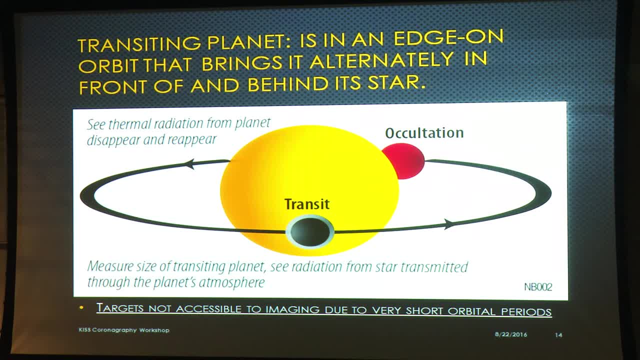 it doesn't help us in imaging very much because pretty much all of the transiting planets they're found in short period orbits And we can't look in that close, you know, inside of an AU generally to be able to get those planets accessed with imaging. 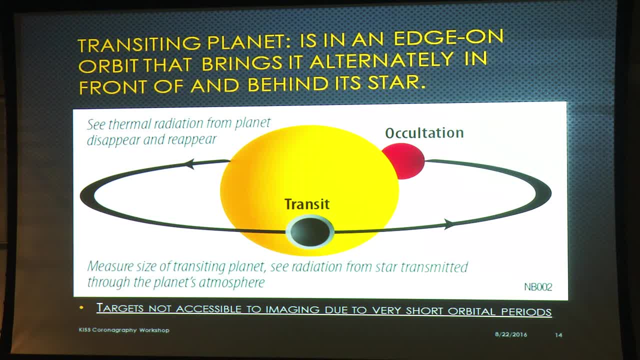 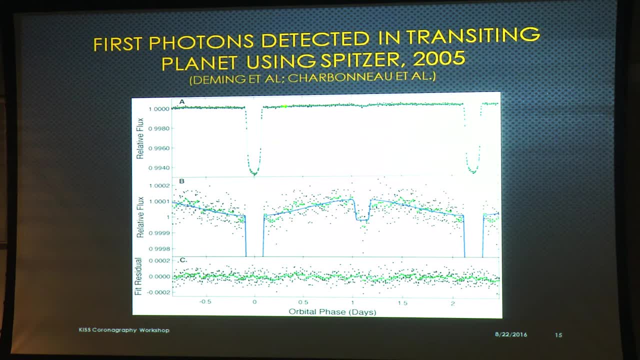 So transits are actually accessed with spectroscopy in a totally different technique, But this shows, for example, a transiting planet passing in front of the star. Then there's a very faint transit here, as the planet goes behind the star and the planet's light disappears. 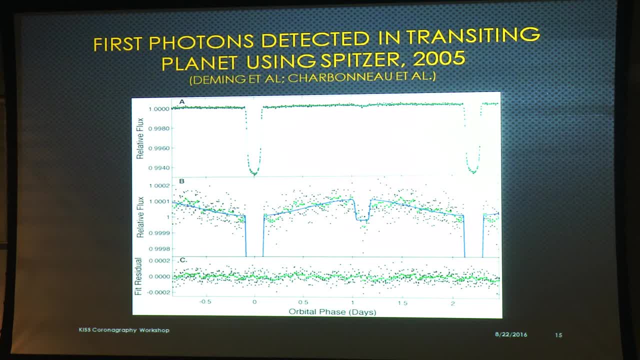 And then it repeats periodically. If you zoom in on this signal on this middle panel, you can then see a little better the secondary eclipse, where the planet goes behind the star, And so that is actually, unless you want to count the brown dwarf planet. 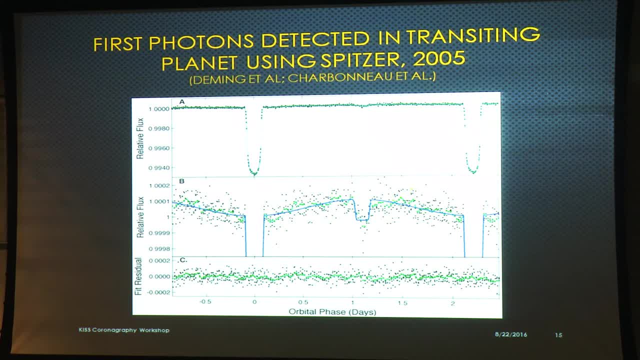 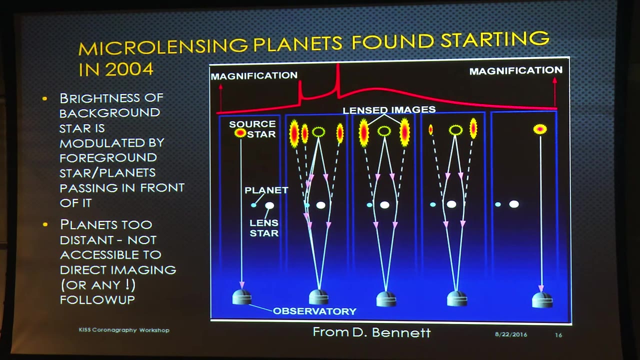 that I showed you earlier. that is really the detection of photons from a planet that was made by the Spitzer Space Telescope in 2005 in two targets. So Spitzer, beat us imagers, unless you like, the brown dwarf planet. So, lastly, in terms of review and analysis, 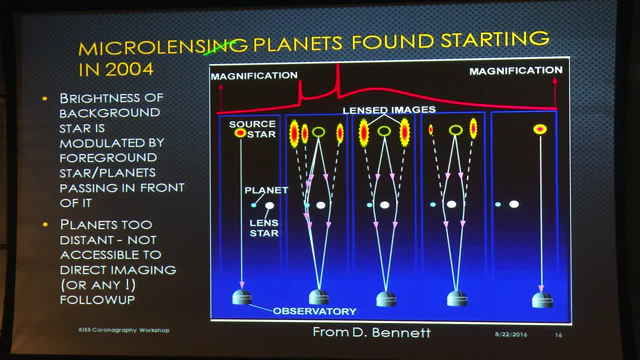 including the other different techniques. microlensing started getting detections in 2004.. And, of course, the technique depends on there being a planetary system in the foreground and some background object that you generally aren't interested in at all, except it's a flashlight. 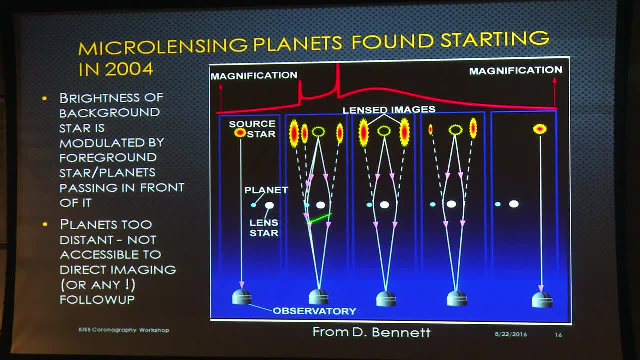 And as that foreground planetary system moves across the line of sight, it can magnify and distort the image of the background star and amplify it And you get these light curves of the star passing in front of the other star and extra little blips from the presence of a planet during the event of passing in front. 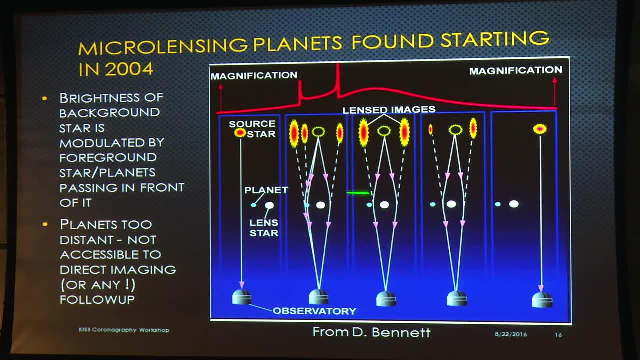 So this is becoming a more productive technique. It's going to be great for WFIRST But again, on imaging, it doesn't help us with targets because these planets are very far away, They're halfway across the galaxy And we can't possibly resolve them with any near-term technique. 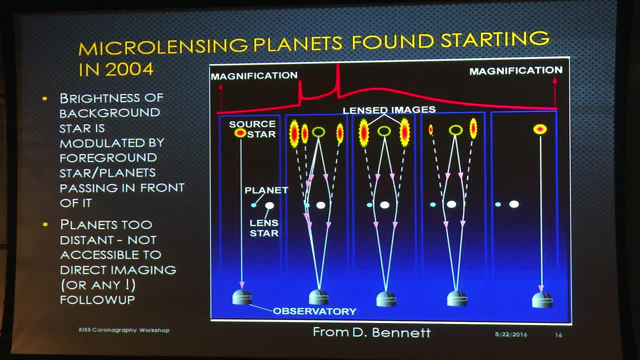 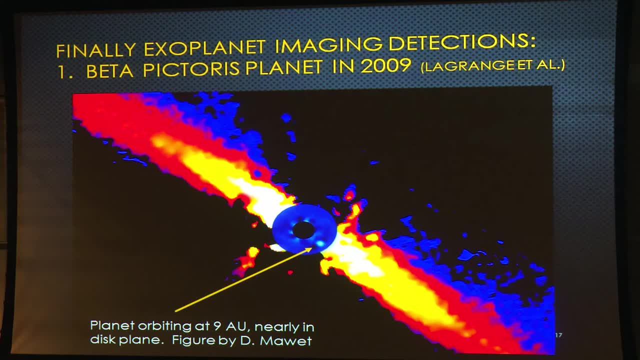 And in fact they're very frustrating because you can't follow them up really in any way at all. once the lensing event has taken place, There's really not much more to do except model it. So we really got to feel we were making progress in the late 2000s. 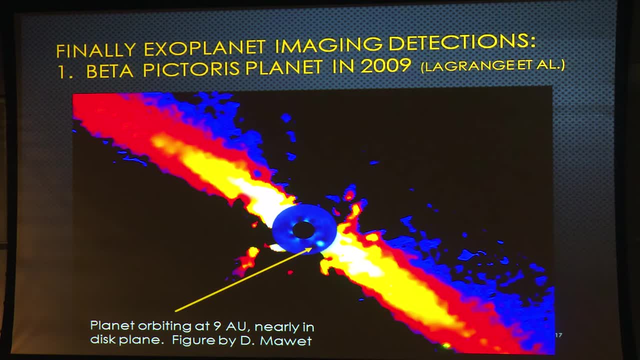 Beta Pictoris disk had been out there for a long time, imaged and studied, And then Anne-Marie Lagrange, in data that was taken a few years earlier but was only processed, well, by 2009,, found an object right in the disk plane. 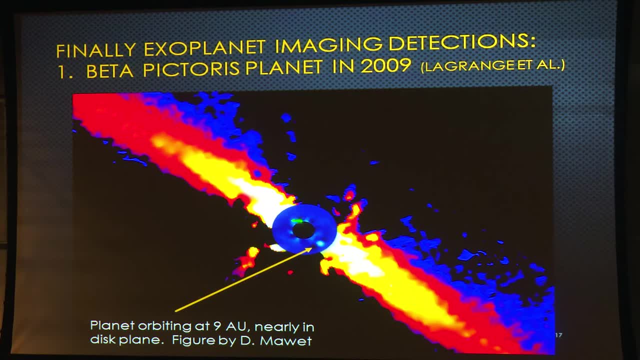 and then waiting patiently for a year, saw it move to the other side of the star, And now this has been tracked very well- the orbit, by including some people in this room, And so the planet is orbiting around nine astronomical units. 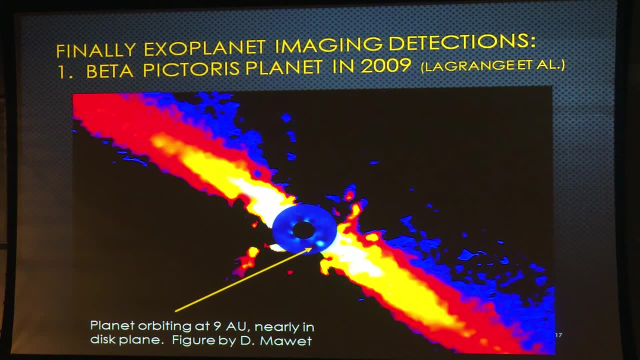 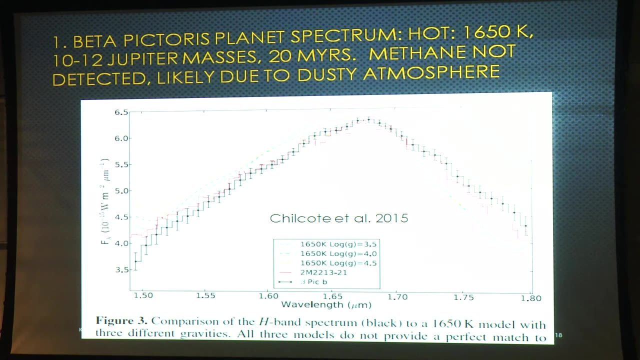 Its mass is somewhere up around eight Jupiter masses, if I remember correctly, And so this is just an outstanding success in terms of showing that a young star has a luminous planet and a very bright disk that's still in the process of clearing. Now, the spectra of these imaged planets is of great interest. So if you look at Beta Pictoris b, the spectrum here in H band shown from G-Pi, Jeff Chilcote's work shows that the planet is extremely hot: 1650 K, as the earlier measurements did. 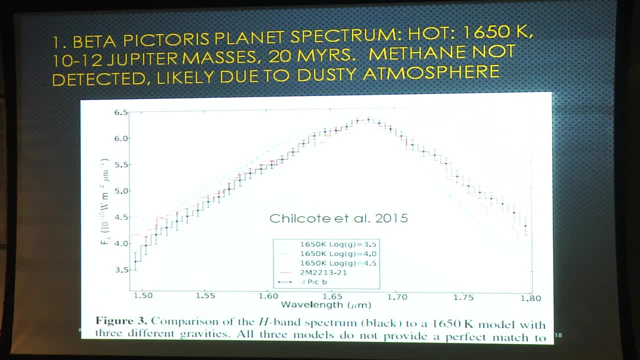 But the spectrum here shows that we're not seeing the presence of methane strongly on the shoulder, on the right-hand side of this hump, like would be expected, And so this is a feature now. of all the planets that are hot like this is that we just don't see the methane feature at all. 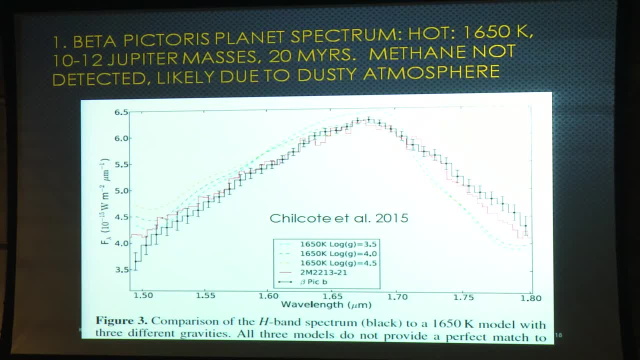 600 K is normally the boundary where you expect to see methane come in for a T dwarf, So this is hotter than you expect for that, And so the methane's absence is also due to the fact that the atmosphere is dusty, as well as to the high temperature. 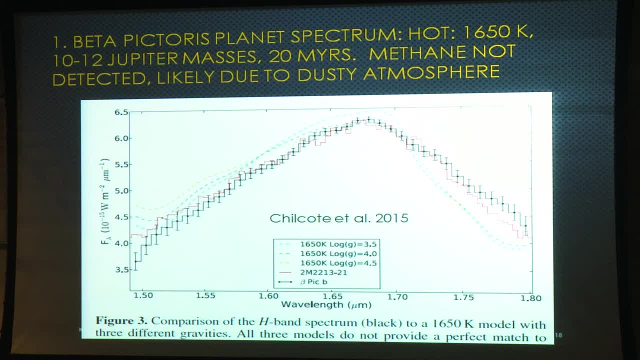 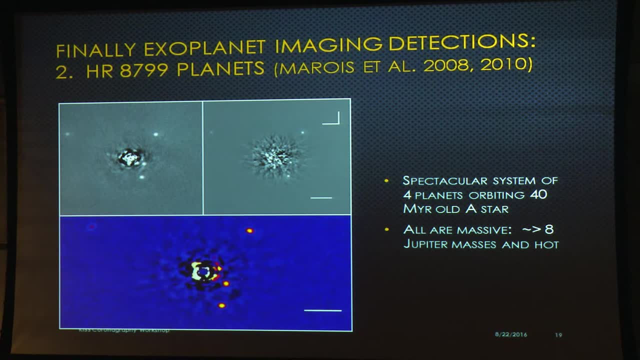 So this is allowing us to interpret the abundances in the atmosphere, especially in conjunction with other higher resolution spectroscopy. So, of course, the really standout system for exoplanet direct imaging over the past 10 years has been HR 8799,. 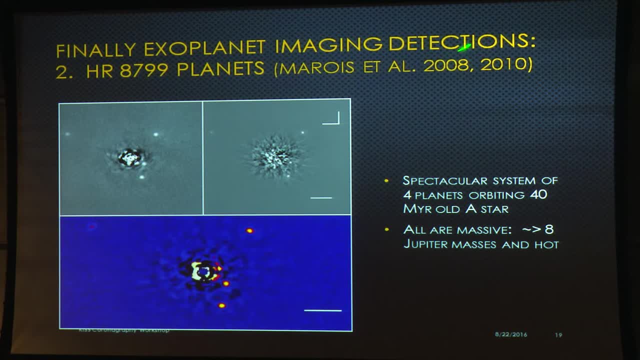 which I think lots of you who work on the system know it like the back of your hand. Here's the images taken by Christian Marois in two different bands in a colored composite showing these four massive planets that are hot, a 40 million year old star. 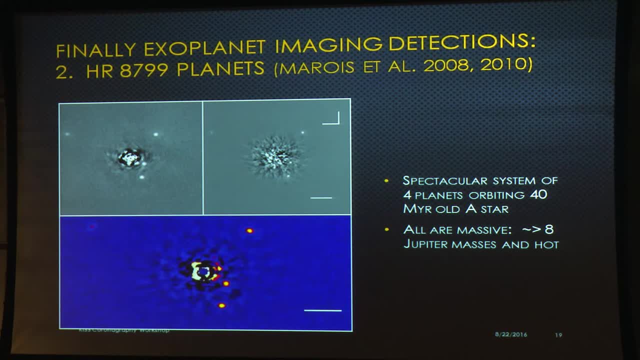 all about 8 Jupiter masses or more, but depending on the evolutionary models as to whether that's really the right mass. And now the orbits of these have started to be tracked pretty well, so we're getting an idea of how coplanar they are. 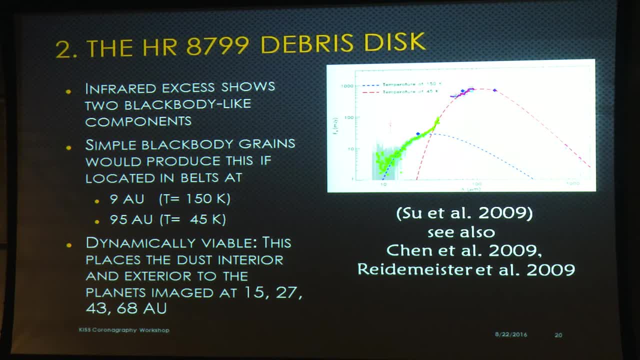 It's almost a face-on system And these planets are like Beta Pictoris in a system that has a debris disk. Now we can't see that debris disk in scattered light at high resolution. It has been seen in low resolution with ALMA and even lower resolution with Spitzer and Herschel. 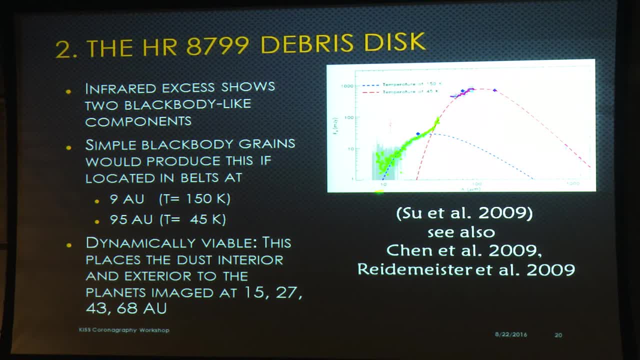 But the interesting feature after you subtract away the stellar spectrum, is that the resulting infrared excess- here in the mid-infrared with Spitzer-IRS and then at the 17 microns and longer wavelengths, it shows that there's two components of dust in the system that are needed to fit this excess. 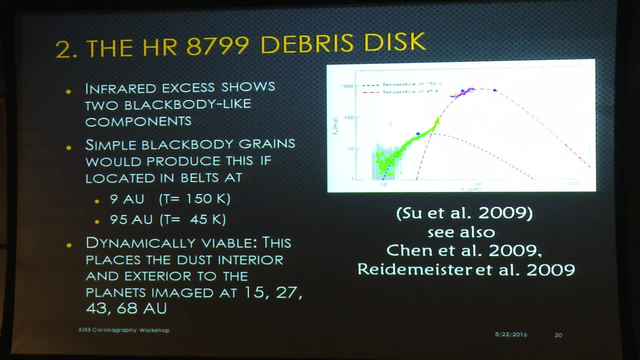 This is a simple model with two black body components, And so one of them is in close, around 150 Kelvin. The other one is much further out, around 95 AU 45 Kelvin. These distances require some assumptions about the grain properties. 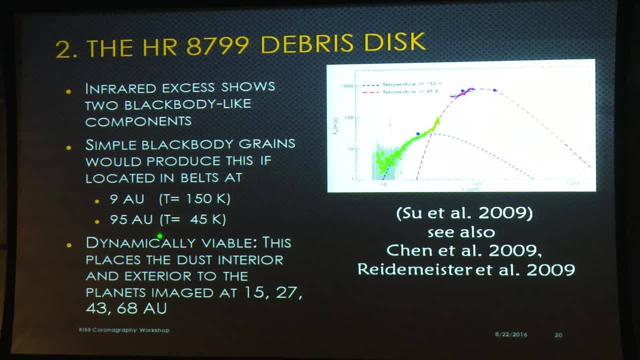 But the nice thing about this picture is that we published this in 2009, after the 2008 detection of the first three planets, but the fourth planet wasn't found until 2010.. And so when it was discovered, thank goodness it was at 15 AU. 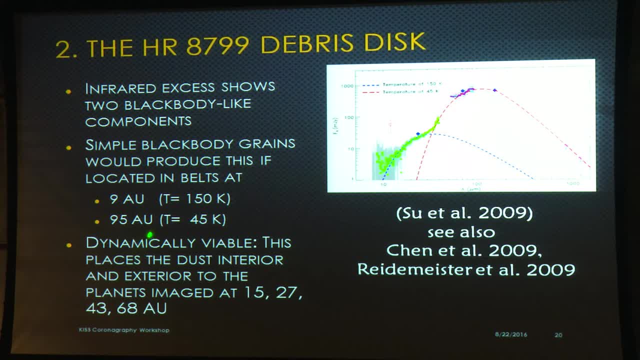 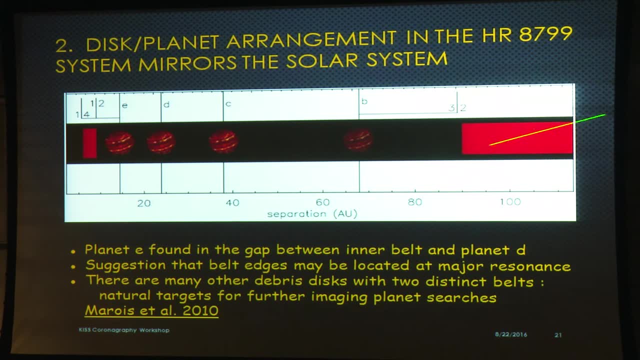 and wasn't sitting where we said the disk would be, because of course the planet would chew up the disk and it wouldn't be there. So we have this very nice picture of an inner disk, an outer disk and these four giant planets much more massive than our Jupiter. very hot. 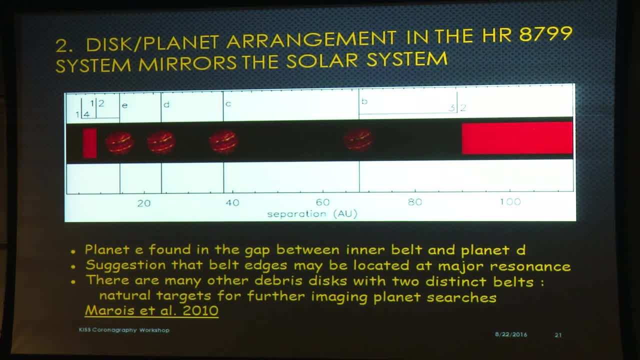 but they're nestled in between these two giant planets And these two disks, just the way in our solar system. the asteroid belt and its dust is interior to Jupiter and the Kuiper belt, and the dust that we assume is there is out past Neptune. 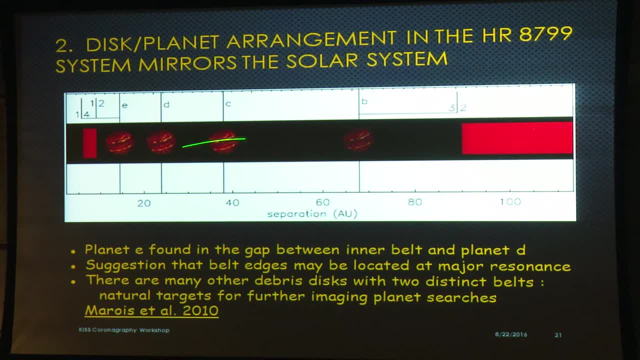 So you can almost think of this naively as Jupiter, Saturn, Uranus, Neptune, four planets in the same gap in the system. So we found through Spitzer studies there are many other debris disks that have two belts in their spectral energy distribution structure. 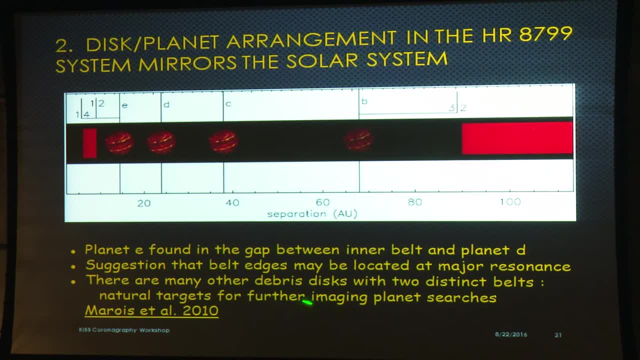 just like HR 8799.. And these are natural targets for further imaging planet searches, And so some of us in the audience are working on that with the Keck folks. Farisa Morales is working on that, and there's VLT observations that are happening to do this too. 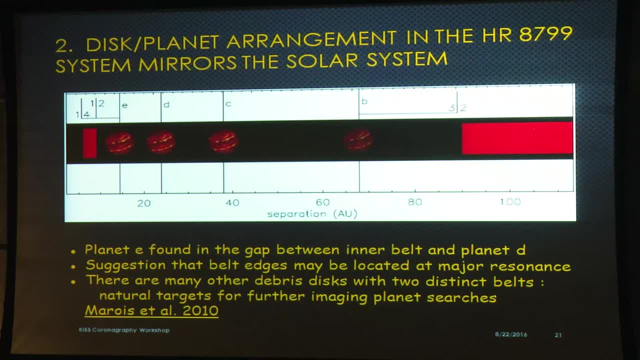 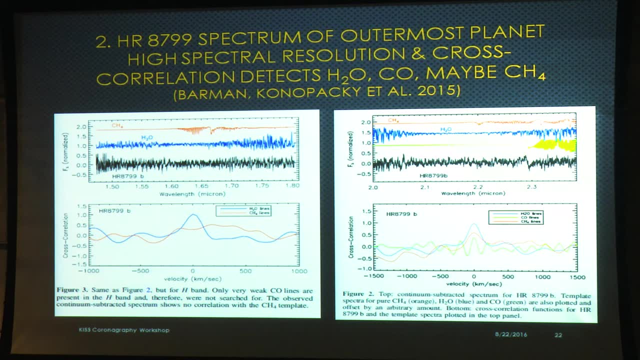 But it's hard to find a system that has got as young as this and it's got as massive- a number of planets as this. All right, so now, spectroscopy of these planets is something that has been a very strong effort, And this is a paper from 2015 that Travis Barman and Quinn Konopacki went and did. 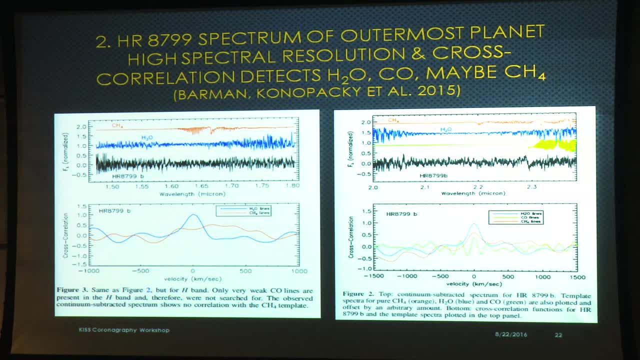 And so here, what they're doing is they've observed, using the Keck Integral Field Spectrograph, OSIRIS, they've measured imaging spectra of the outermost of the four planets, HR 8799b, The outermost one, is farthest away from the glare of the star. 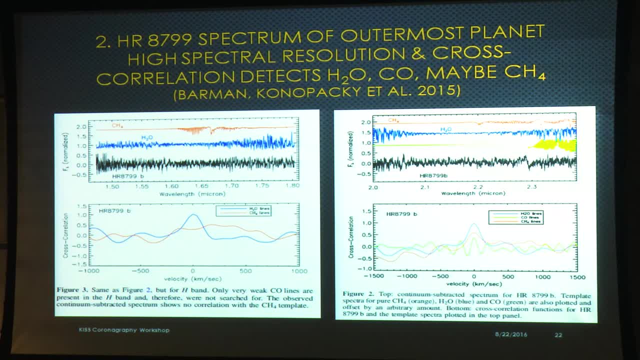 so it's easier to get a clean spectrum. This week, I hope, we're talking about how to clean up our spectrum much closer in, which remains a challenge. And so here's the spectrum of this outermost planet, from 1.5 to 1.8 microns, and also at 2 microns. 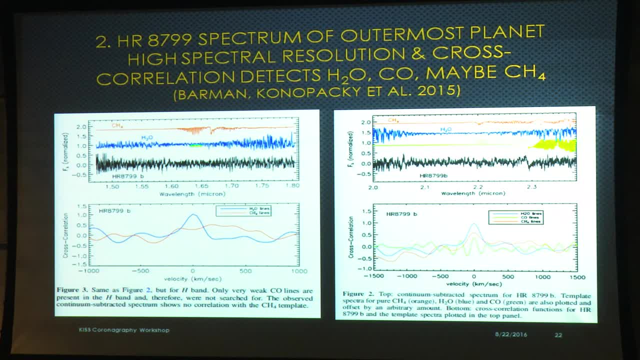 And so the technique that they used- that Quinn first did in 2013- is to correlate the spectrum of a molecule of interest at the temperatures that you think are appropriate for the atmosphere here. correlate this with that and see how strong a cross-correlation you get. 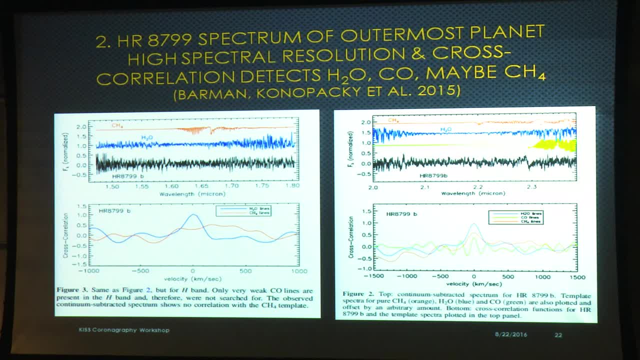 And so if you see a peak around zero velocity, that means that this spectrum, the species you were checking for, is significantly present in the spectrum, And this gives you the advantage of, instead of trying to find just one absorption line to see, the planet is there. 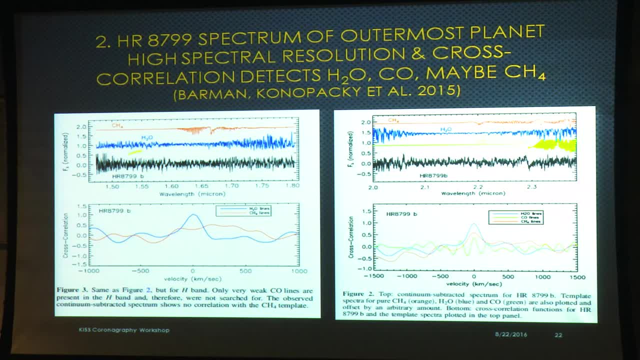 you can use all the different molecular bands that are present at all these wavelengths, you can use a signal from them, And so that lets you pull out a much fainter level of presence of that material. So here in planet B, at this wavelength range, 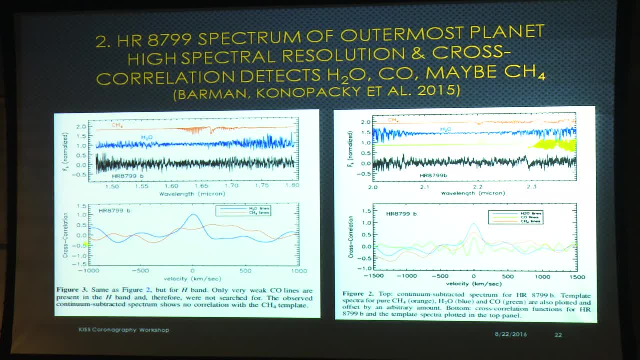 water is indicated and really the methane doesn't have much of a peak there, maybe a very weak one, because that's consistent with a lack of methane in the Beta Pictoris B planet. But this paper also shows the same analysis being done in the 2 micron region. 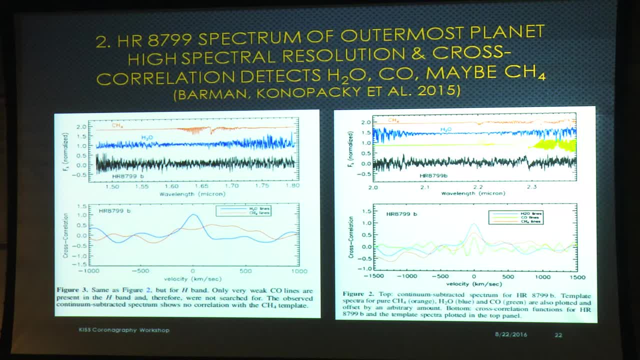 And so in this region, carbon monoxide is showing up pretty well at this little jump here, And the methane seems maybe to be showing up. this is being shown here on the orange. it's a more significant peak than it is there, And then I'm not quite sure how. 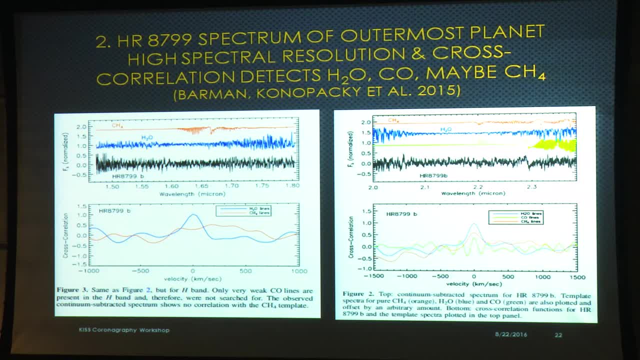 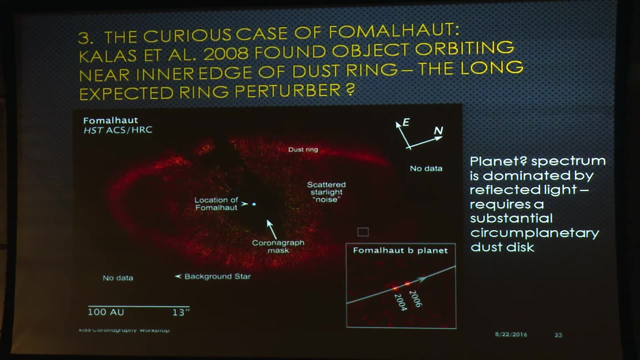 the CO is. I guess that's significant, but it's oscillating around a lot, So this is the best opportunity to dig out the composition of these planets. is this correlation method Alright? so then, the third of the planets that came up back in 2008-2009? 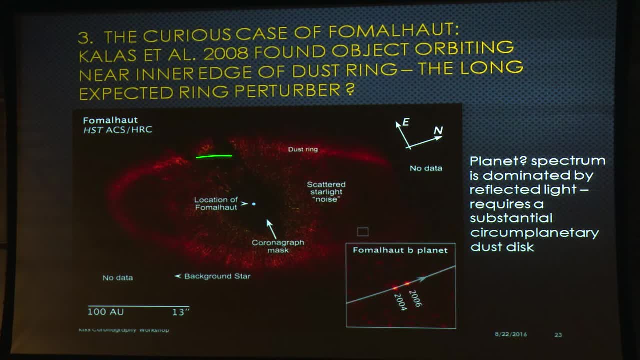 was the Fomalhaut B object. This is the original HST discovery image. Fomalhaut is a bright nearby star that has a dust ring around it. it's appearing elliptical mostly because it's inclined, but it's also slightly offset. 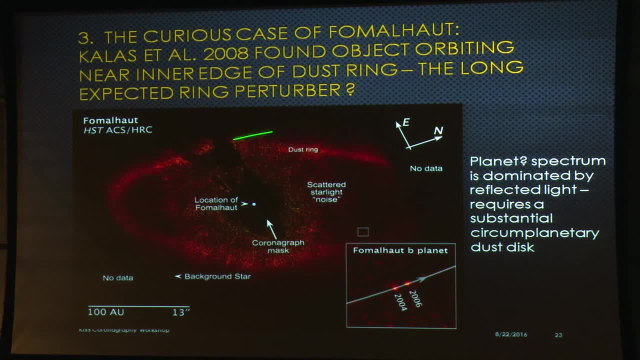 the center of the disc is offset from the star because of an intrinsic eccentricity of the dust ring. In order to make that eccentricity and maintain it, theory says you need a perturbing planet close to the ring inner edge. And so, when this popped up, 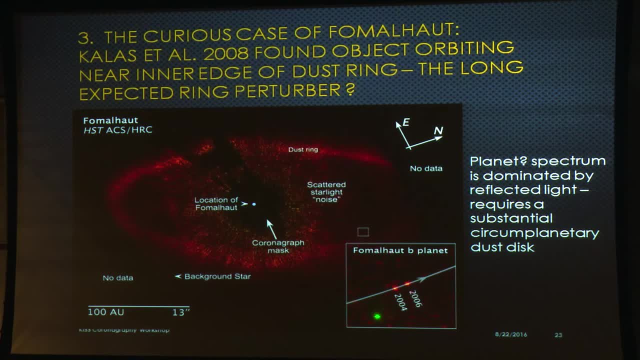 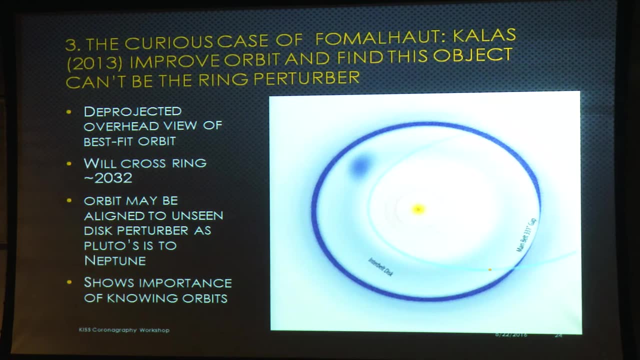 the team that I was on. we concluded- hooray. we found the object that is causing the disc to be eccentric and sculpt the inner edge. But more data shows the situation is not as straightforward as that. That Paul Callas analyzed the same system again in 2013,. 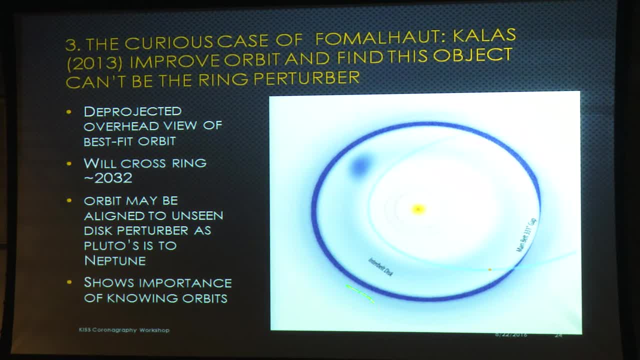 using additional HST data and deprojected the orbit the best fit orbit. there's a wide range of orbits allowed, but this is sort of the median best fit orbit And the planet next to the ring is actually on an orbit that has to be going out and crossing it. 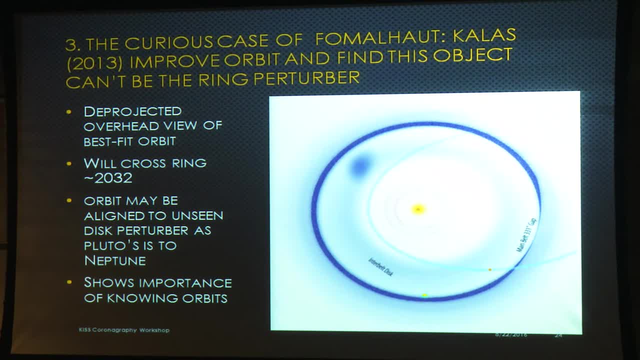 And that's not what should be happening. if the planet was sculpting the ring, it should be just tracking the inner edge with the same eccentricity that the ring has. So this is not the perturber that's creating the ring. it's some kind of object from the outer belt. 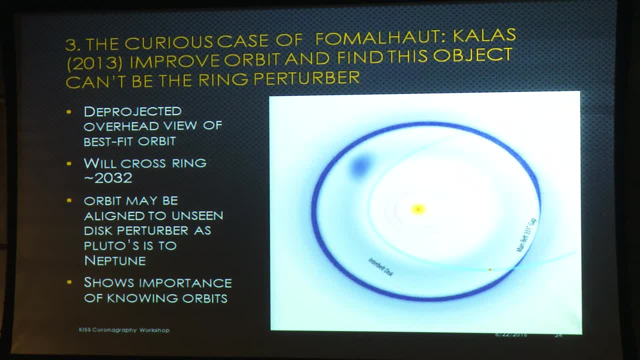 an interloper that crosses it. In my mind this has always been analogous to the way that Pluto crosses Neptune's orbit: that Neptune actually controls the dynamical state of Pluto and they never get a chance to collide with each other. So I'm kind of always liked the idea that the planet that we can't see 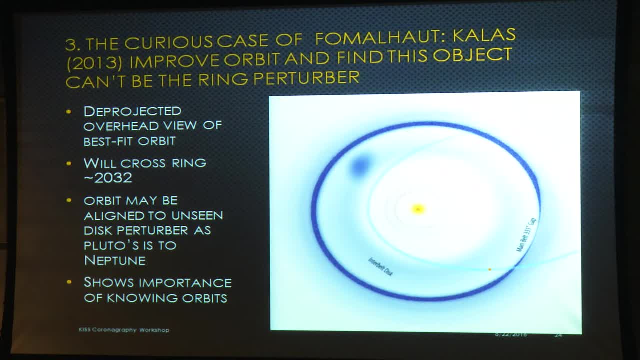 that's sculpting the ring is dynamically controlling the eccentric object here. that would be the analogy to Pluto, But this shows that you can't really interpret what you're seeing in terms of disk interactions, unless you've got the orbits figured out. So another really weird thing about this object is it's just ridiculously bright. 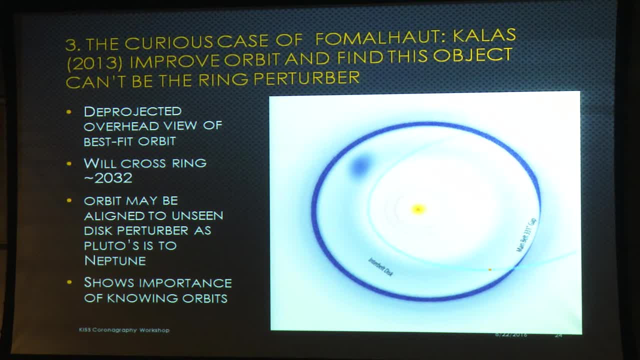 It's so bright that it has to be reflecting the light of the star with something 10 Jupiter radii, which theory says you could never have something that big. So the interpretation has always been that there's a lot of dust around this object. 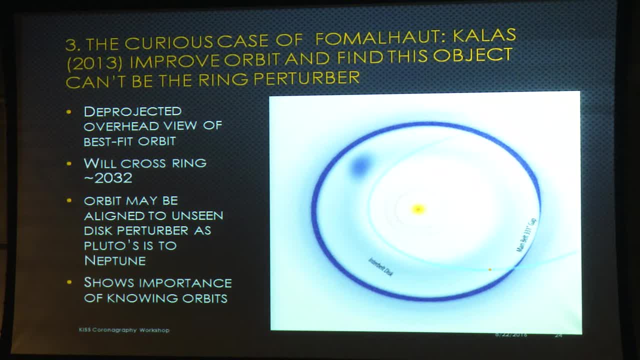 And because I was on the original paper, I'll always defend the possibility that this is still a planet, although I know many of you in the audience are subscribers to the theory that this is just a bunch of dust from a collision that took place. 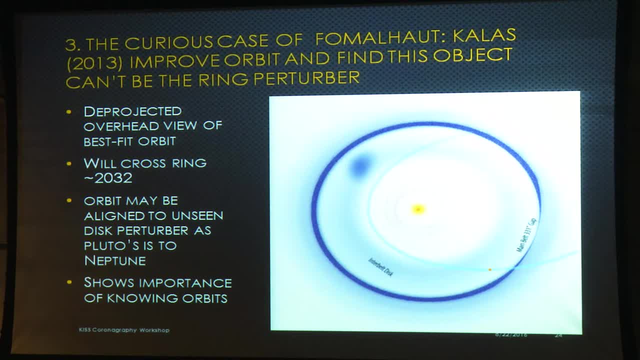 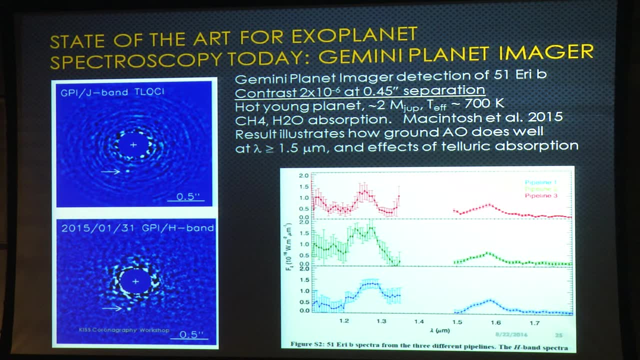 But the argument against that is that it doesn't look very extended like a dispersing dust cloud, although the signal to noise is too low to really tell. So where we've gotten to today in these direct imaging searches, there are other examples I could show. 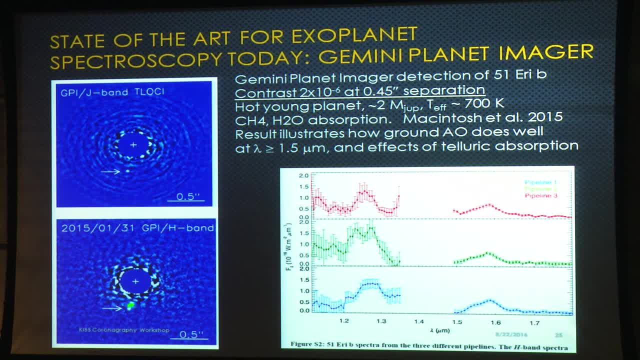 but this is the highest point of performance, result of direct imaging for an exoplanet companion, And this is the GPI result for 51 Eridani b, another young moving group star, And so the planet is visible here and here You can see all these features that are leftover residuals. 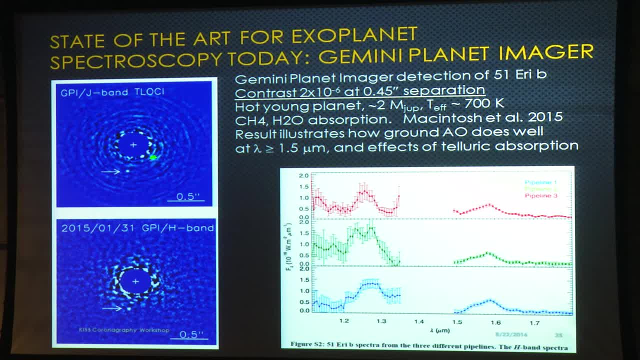 of the subtraction of the starlight. So here it is at J band, Here it is at H band, And then Bruce McIntosh's paper plots those spectra that they get from their data cube here And the first thing you notice is that 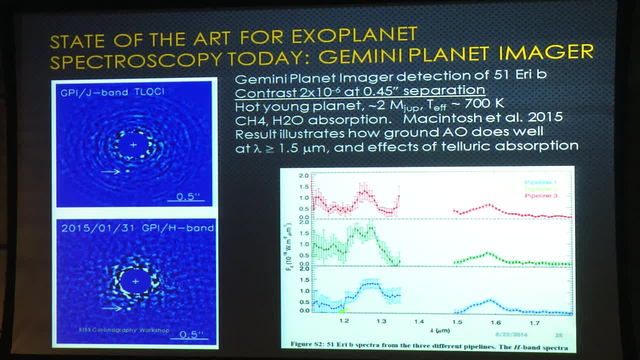 at shorter wavelengths it's harder to get good adaptive optics correction, so there's bigger error bars on all the spectral points And then at longer wavelengths, out here in H band things are much more under control, But nevertheless the difficulties that he has processing this. 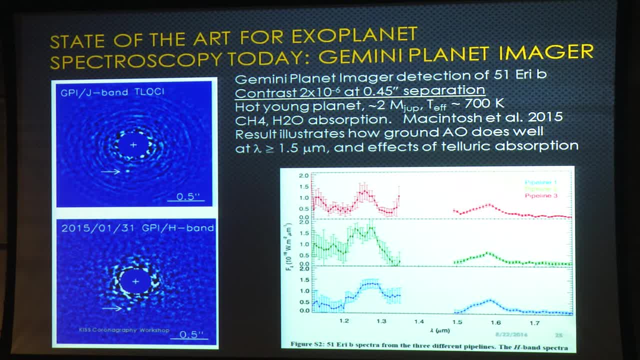 are something I hope we're talking about at the meeting this week, which is that Bruce thought it was necessary to process the data with three different pipelines, different analysis methods, and see if the spectral features came out consistently between them. And so, in some ways, yes, 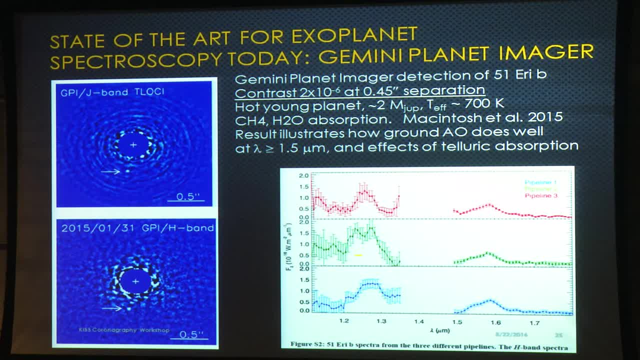 In some ways. no, I mean, this bump over here isn't really present over there, And then there's other things that are happening within the noise level. So this is something there's still progress to be made at, But the great thing about this detection. 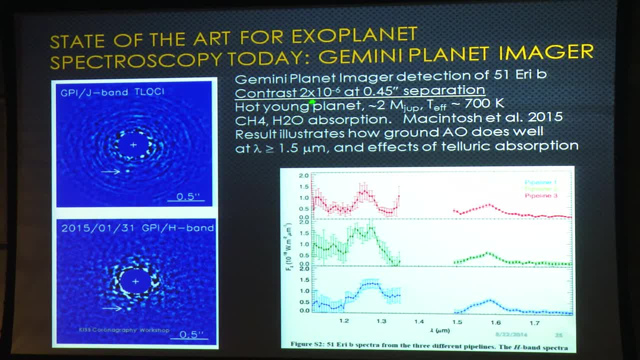 is that it's at 10 to the minus 6 contrast after subtracting off the stellar halo And it's at half an arc second separation. So this really defines the state of the art in high contrast imaging in the near infrared from the ground. 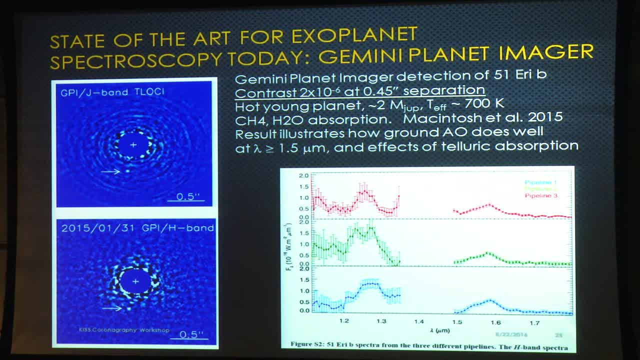 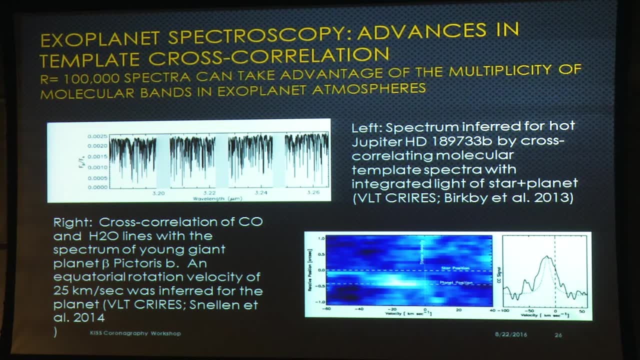 And it also shows that we want to look at longer wavelengths, like H-band, and longer to get our best results, at least with current AO systems. So the correlation spectroscopy method I showed you applying to the abundance analysis earlier on can also apply to both the spectrum of transiting objects. 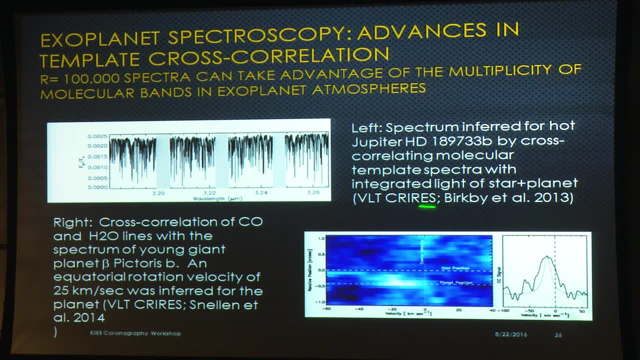 Well, in this case, I think they didn't need to use the transit aspect of it. This is a known radial velocity planet And it also applies to analyzing the dynamical state of the planet. So, Snellen et al in 2014. 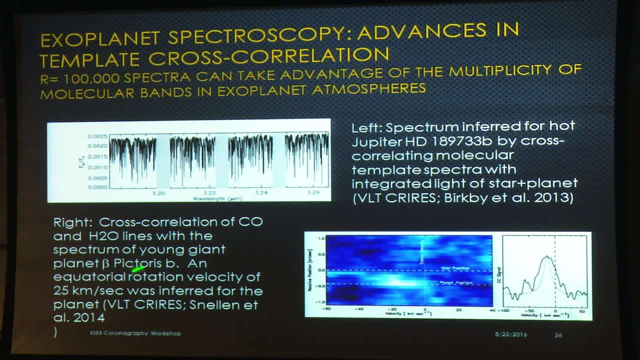 took correlation spectra of beta pictoris b, And now they're not just looking at the fact that there's a nice bright peak here of their molecular correlation, but this peak has a width that is broader than the instrumental width, And these folks interpreted it. 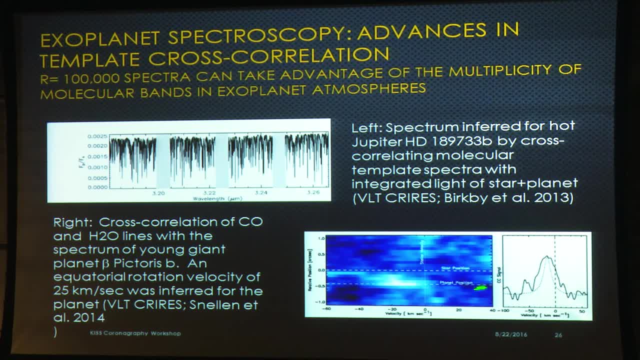 as rotational broadening of the planet. So we're actually able to see the spin of this very young, hot planet through this method, And it's a 25 kilometer per second equatorial rotation rate. v sine i was indicated at this. 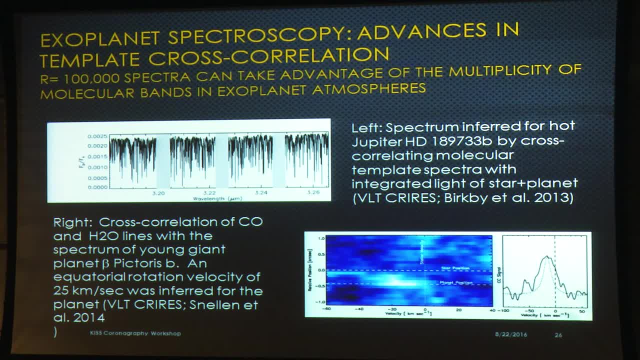 So this is pretty interesting that you're able to do this. The contrast is 10 to the minus 4 of what they've been able to do so far, But I don't believe any coronagraph was used for this observation, So doing this again with a coronagraph. 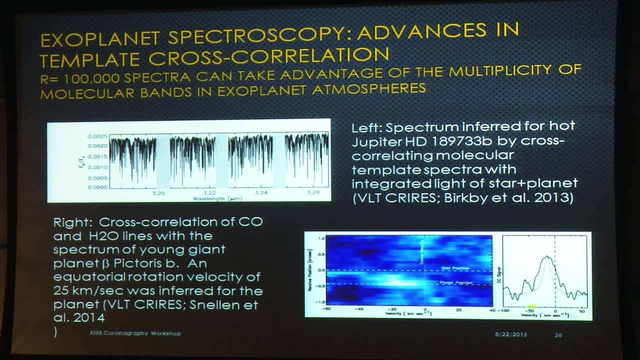 to suppress the speckles. it might be interesting to see how much fainter we could go. So I look forward to somebody going and picking a dimmer target of 10 to the 5 contrast or 10 to the 6 contrast and trying to repeat both the spin analysis. 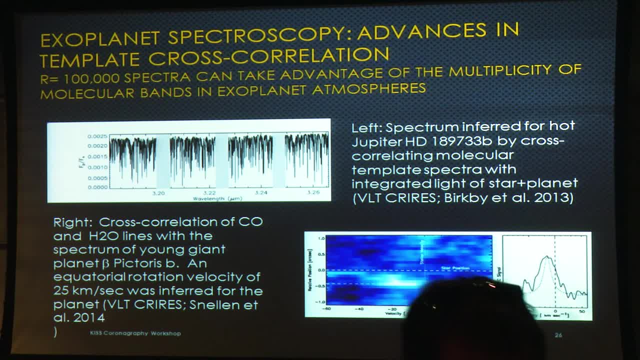 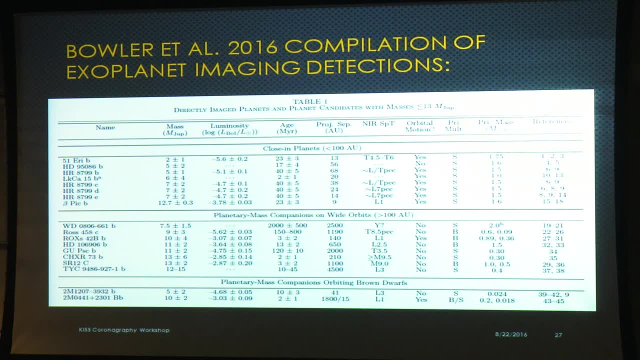 on other objects and then this atmospheric abundance analysis. So it's a really great review paper that you should have a look at if you hadn't yet. Brendan Bowler, who used to be here, he's now at Texas. he has a paper compiling the results. 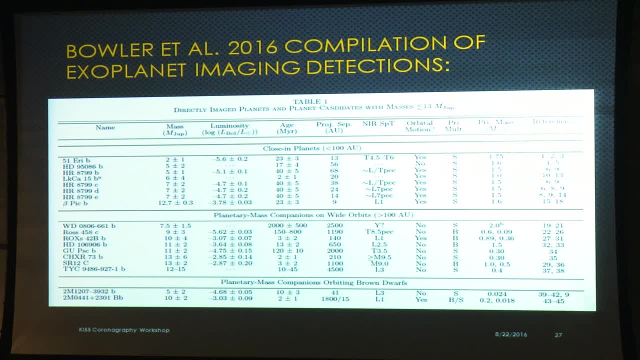 of many different direct imaging surveys that were done at all observatories around the world by different groups, And it's a really good state of the art paper for early 2016 on what we know about these objects. There's a whole other table about planetary mass companion candidates. 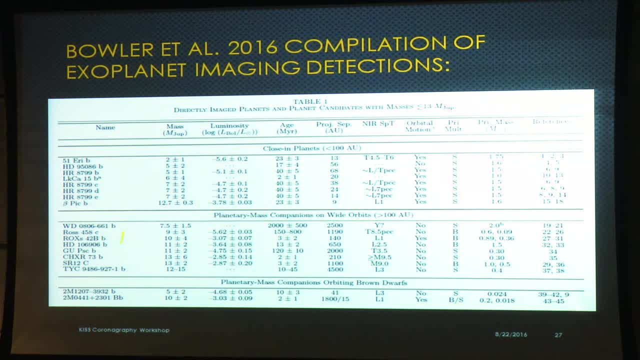 that I didn't include here, But these are the ones that are deemed relatively confident. So here's 2MAS 1207, a planetary mass companion around a brown dwarf, and there's another one that's known here. Here are the more famous objects. 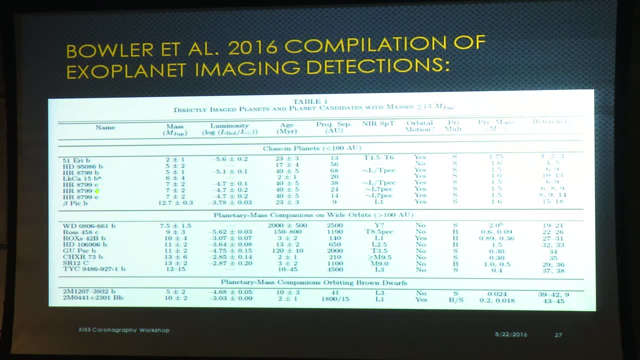 I just discussed 51, Airy 8799, all four of its planets, Beta Pictoris, B, A couple others I didn't mention but are also very interesting. calcium 15 seems to be an example. This is the Cretan protoplanet. 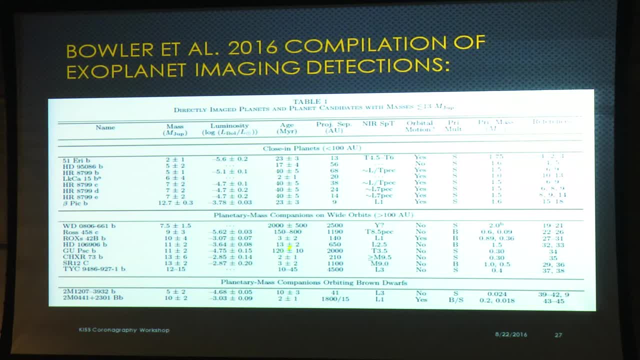 And then, while these are close in, these are on much wider orbits. So it's unclear, there we go. projected separation, So it's unclear whether these are formed in a disk or whether these were formed on the collapse, like a binary star took place. 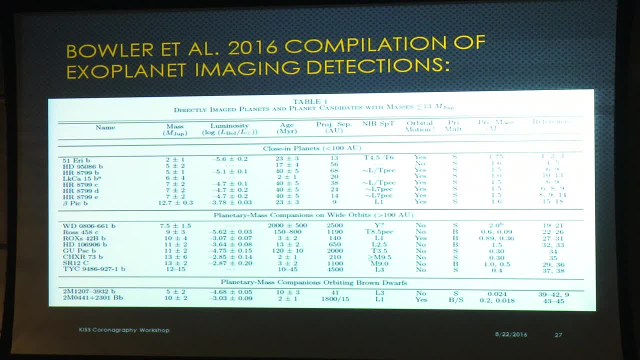 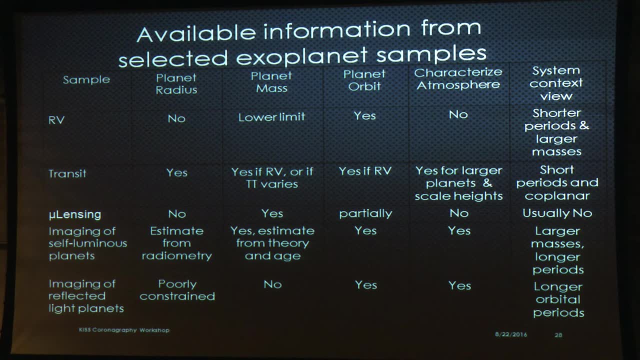 So the physics may be different between these two samples. So, combining together imaging, radio velocity, transit, et cetera, how do these different methods enable us to constrain what we're seeing? Well, the quantities of interest are like the mass and radius of the planet. 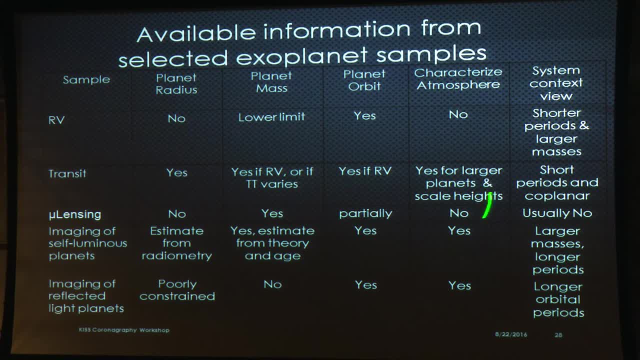 what its orbit is, of course, the spectroscopy of the atmosphere and the context for the planet. Can we see everything else in the system or not using these? So radio velocity is doing well on the planet mass and very well on the orbit. 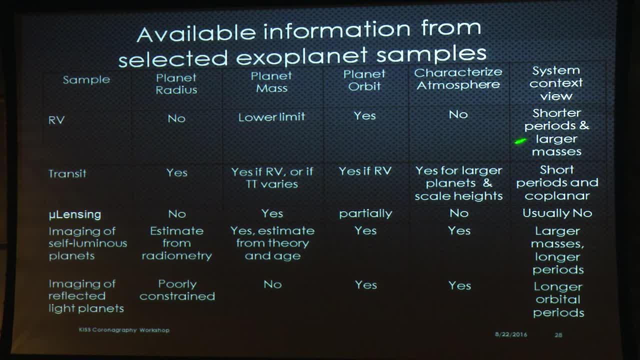 It doesn't give us any atmospheric information and we can only see the closer in planets that are more massive, Then transit observations. their big advantage is they give us the radius of the planet and if it's also detectable with radio velocity. 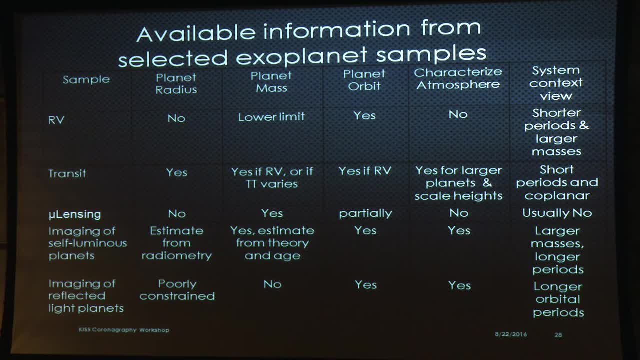 they give us the mass. There's going to be a big intersection of these two with the upcoming test mission. Unfortunately, those will all be planets we can't image. And then microlensing, you know, is getting information on the mass somewhat. 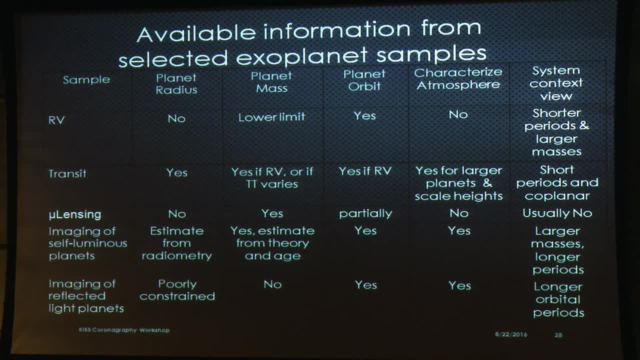 the orbit somewhat, but otherwise no on these things, And ground-based theory is doing much better on the planet radius and mass than imaging of planets in reflected light, which is the higher contrast future of the field, I think, And so both of these are subject. 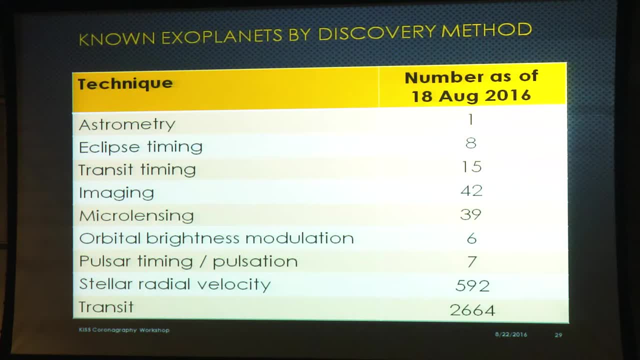 to seeing longer period planets. So what's the count? How well are these different methods doing? How well is imaging doing compared to everybody else? So the results here are that astrometry, according to the NASA exoplanet archive, has one detection. 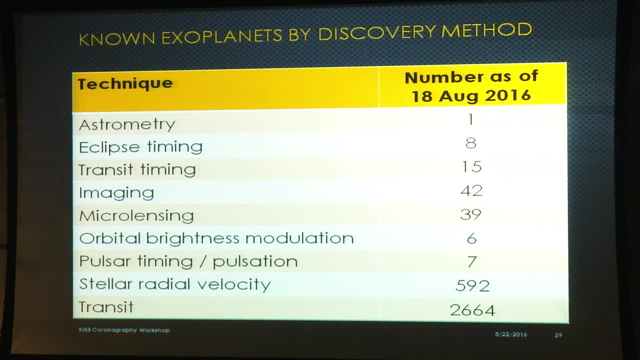 I should have gone and looked in and figured out what that was, because I didn't think there were any. But you can see, imaging has only got about 40 objects, including candidates, whereas you know radio velocity is much, much higher. 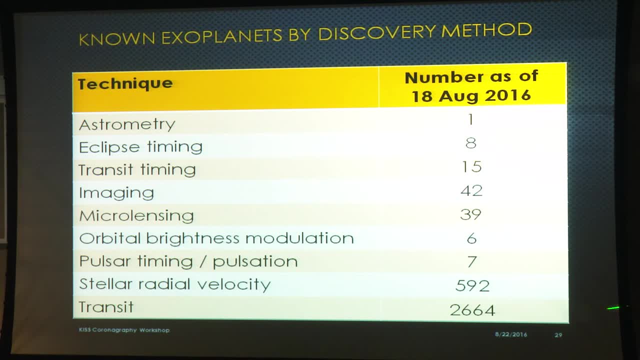 And of course transit is doing hugely well thanks to the Kepler mission. So we don't have a lot of opportunity to intersect imaging with things. The best chance is with radio velocity. but we can't really do that in any way right now with the contrasts available to us. 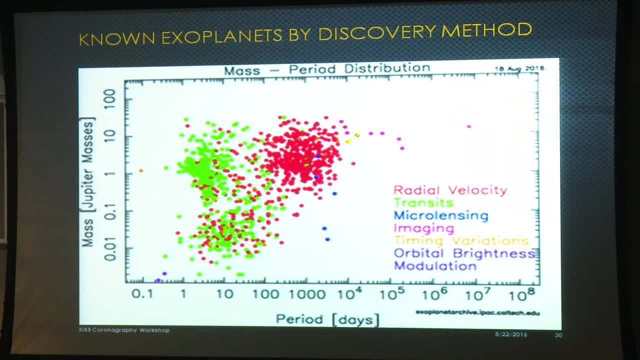 So now, where are these planets distributed? Here's imaging- pink off to the side up here: Wide separations, larger masses and only in very young hosts. And transit is over here. Radio velocity is seeing things that are at a few AU typically. 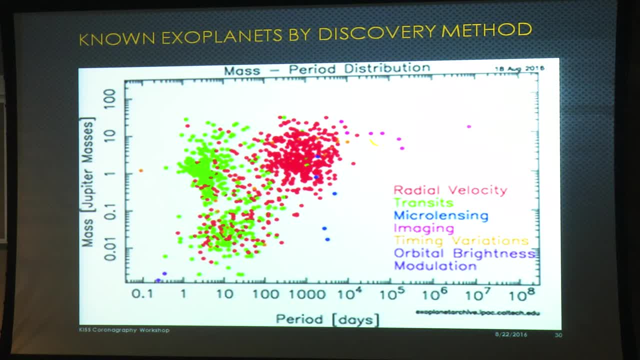 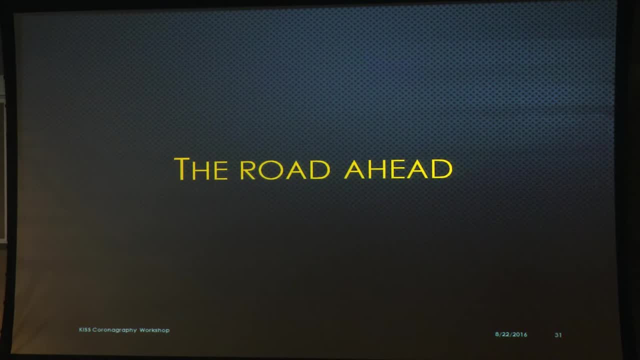 And so, unfortunately, you know again, you can see the fact that these samples don't intersect. really, that imaging has got this outer region probed and not the inner. Okay, I've got about 15 minutes left, So I want to talk about. 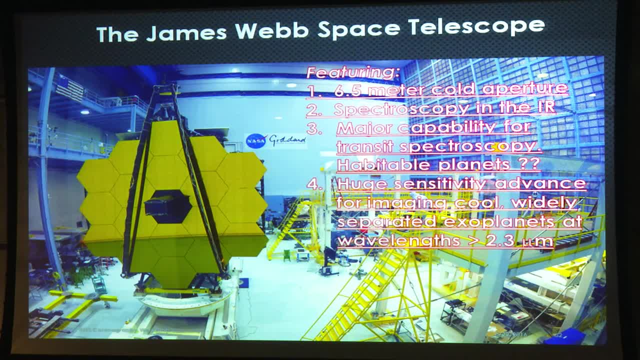 where things are likely to head. So the biggest thing coming is the James Webb telescope. It was a great thing to be at Goddard when that was being put together and go look through the clean room for once in a while To see things like this. 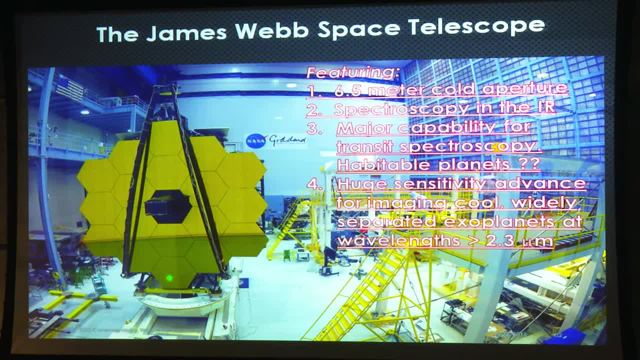 although this day I wasn't there, darn it. And so the great thing that JWST is going to do is transit spectroscopy, which I haven't really talked about, And if you go back, say five or 10 years ago, 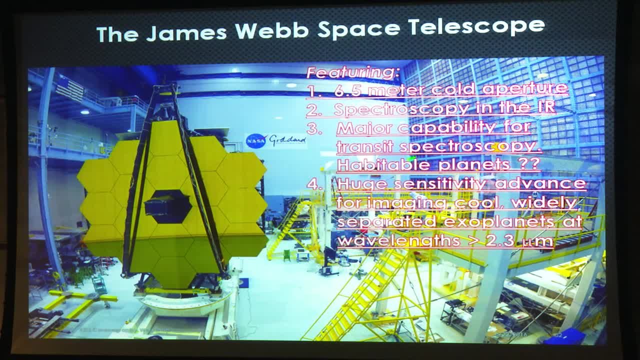 there was excitement about the transit spectroscopy extending down to habitable Earth-sized planets. People are a little less optimistic about that. now I'll get into that And for imaging it's going to have trouble looking in really close but it's going to be really sensitive to cool planets. 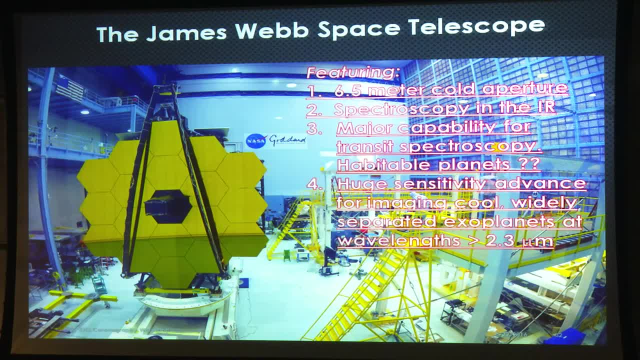 much more than any ground-based observatory is, because up in space, without the sky background, it'll be able to see widely separated companions. Unfortunately, as you'll read in Brendan's paper, the frequency of widely separated companions is low sort of 1%. 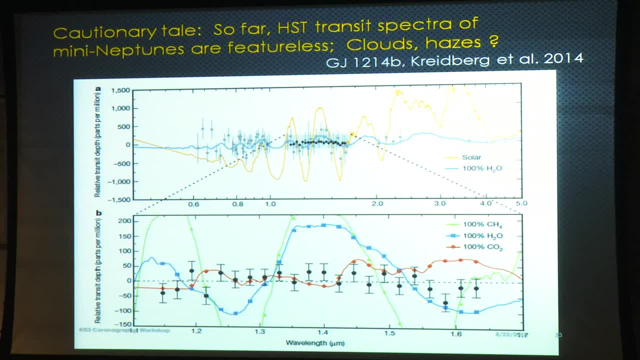 It'll be hard to do lots of surveys with JWST looking for things when the frequency is that low. So for transits, it's instructive to look at recent results from Hubble. This is the so-called super Earth. It's really a Neptune. GJ 1214 b. 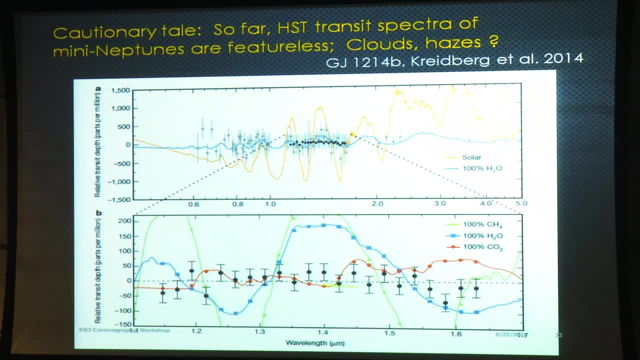 The data is shown here in black points and basically there is no transit spectrum feature that is seen. It's consistent with a flat line. These compositions of water or of methane here are clearly ruled out by the data, So it seems like transiting planets are tough. 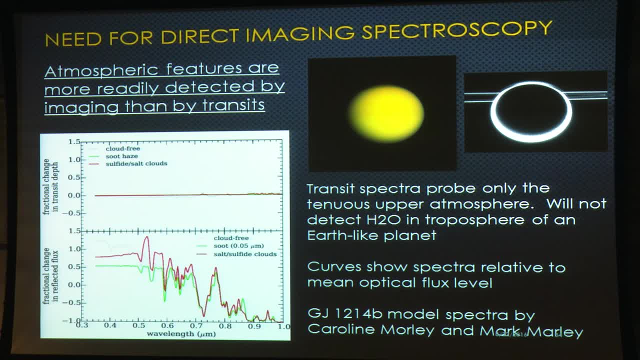 when they get down to be like super Earth-sized or mini Neptune. Basically, what's happening is in transit. you're seeing this kind of situation. This is a Cassini image of Titan, the light passing through the upper atmosphere. So that's just not as much light as you could get. 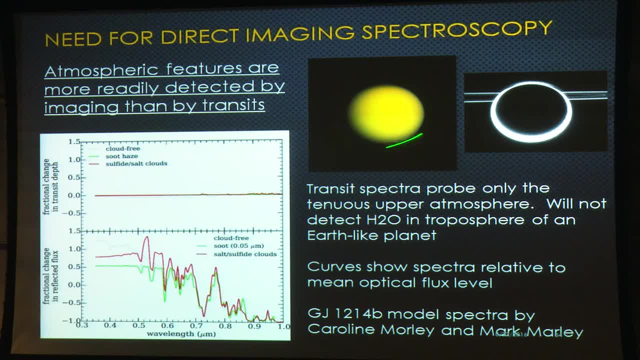 by reflecting off the surface of the moon, getting the full disk illumination, And models show that in transit you really could have situations where you don't detect any features at all. but the exact same model in reflected light produces huge spectral features. So this is encouraging that transits. 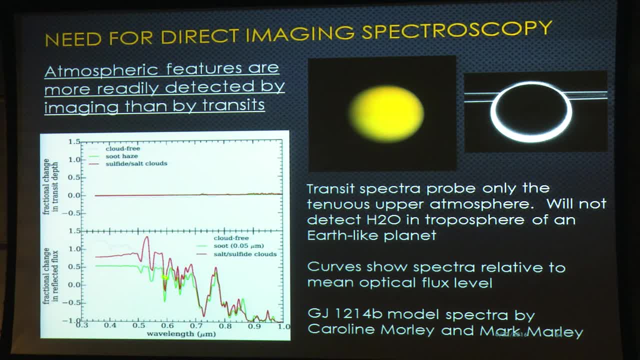 are not going to clean up the field and leave nothing for direct imaging to do, And so this is the you know the future is to do measurements of those features there, And of course the transit not just has that little limb to look at. 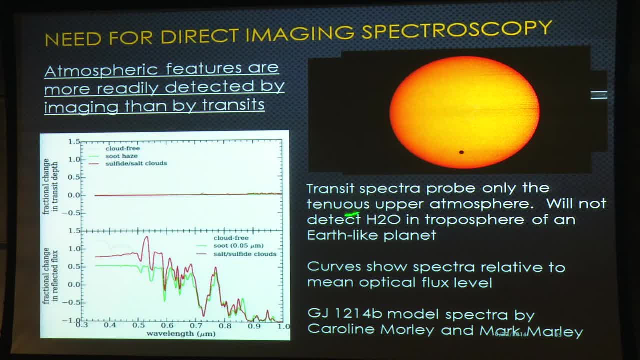 but it's combined with the light of some gigantic stellar signal, as shown here in the transit of Venus. So I'm confident that JWST is not going to own spectroscopy of exoplanets, that there's lots for imaging to do. This is a simulation of transit spectroscopy. 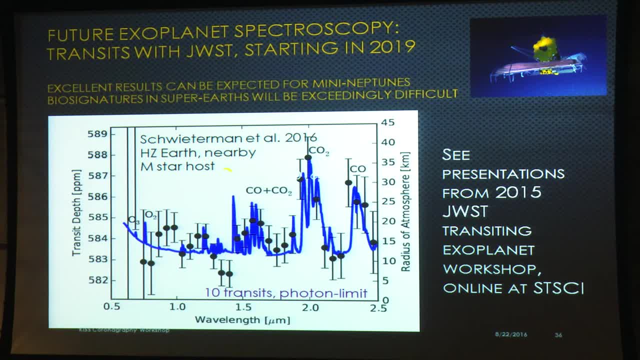 with JWST around, you know, a habitable planet in an M-star host of those favorable situations, So with 10 transits, if there's no systematic errors, they're just not really picking up the oxygen features over here, And they might be picking up these CO features though. 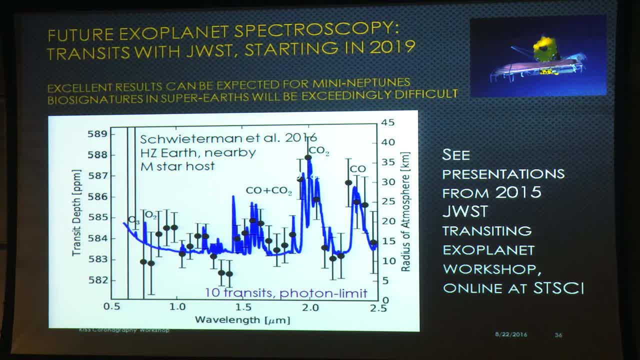 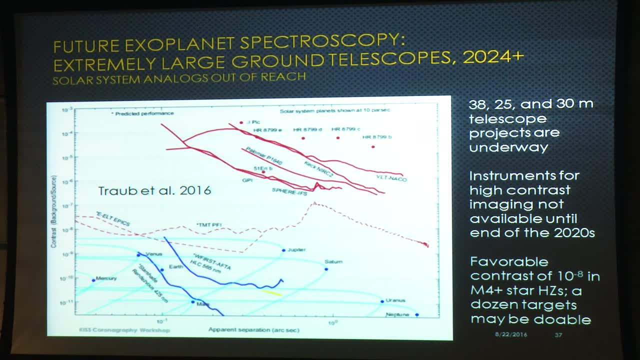 So there's great things to be done in transit. We wish them all the success, But I think again they're not going to put imaging out of business. Okay, let's look at now at the high contrast imaging missions that are coming, we hope, in the future. 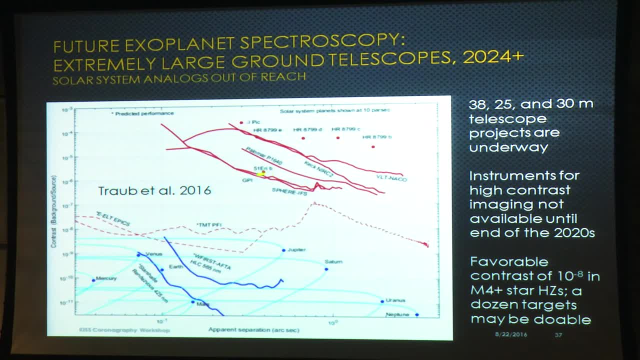 The first of those is going to be WFIRST. Here's where we are right now with the GPI detection of 51 Airy B. Here are our early, easier detections, And our solar system is so far down here in contrast: 10 to the minus 10 or so. 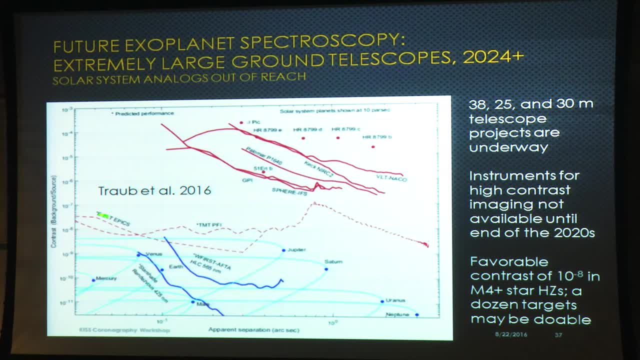 that there's this huge gap that we have to cross. There are estimates of the EELT and the TMT performance to come, So we hope to see that that performance realized. But even if it is, it's not going to get us down to Jupiter-like planets. 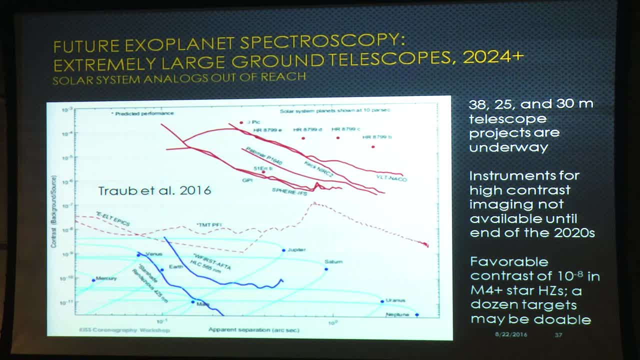 in our solar system or close to Earth's. in terms of this direct imaging technique, The correlation spectroscopy technique has to be figured into this, and it's limits are not known to me very well yet. All right, so WFIRST is a dark energy mission. 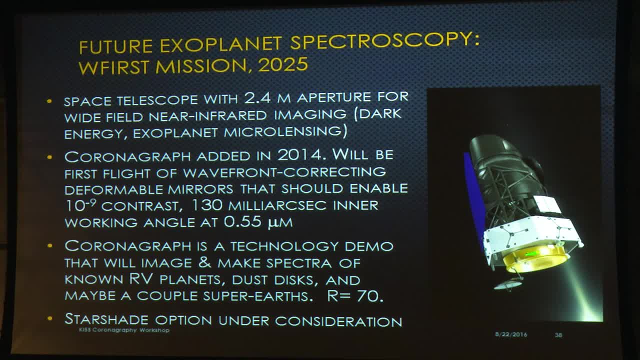 that NASA has just started. It's going to launch in 2025 or so. It has a coronagraph added to it. It will be the first time we can fly in space. A wavefront correcting coronagraph with deformable mirrors should get someplace close to 10 to the 9 contrast. 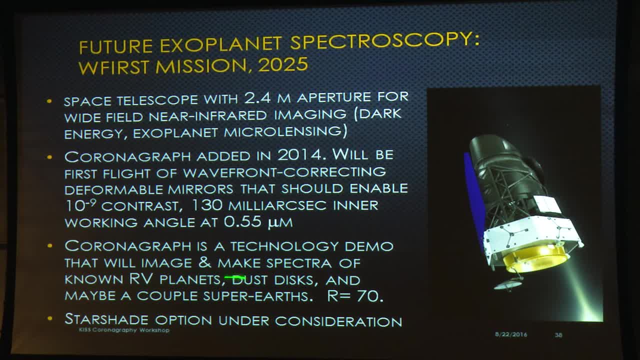 And it'll be a technology demonstration to make sure that we're ready to do a more exciting mission in the future: to do habitable zone planet imaging. If it's very lucky it might get to super Earths. Instead it's just going to do known radial velocity planets. 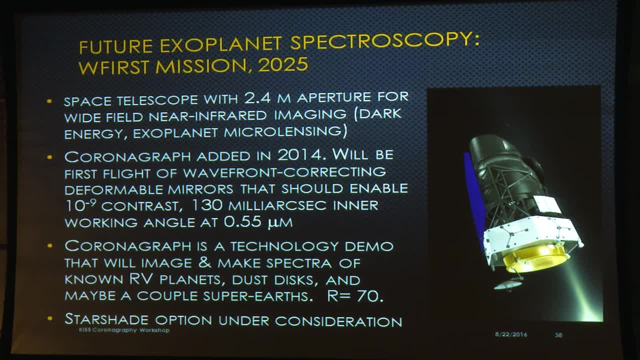 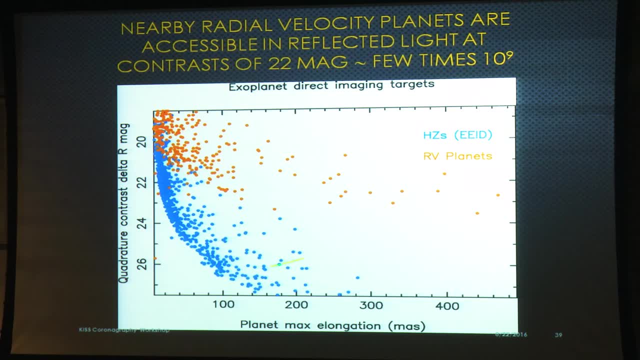 And we could talk later about the star shade option, which is being discussed but wouldn't be acted on until the 2020 decadal survey gets to vote. So if you look now at the known RV planets and then nearby stars where their habitable zone lies, 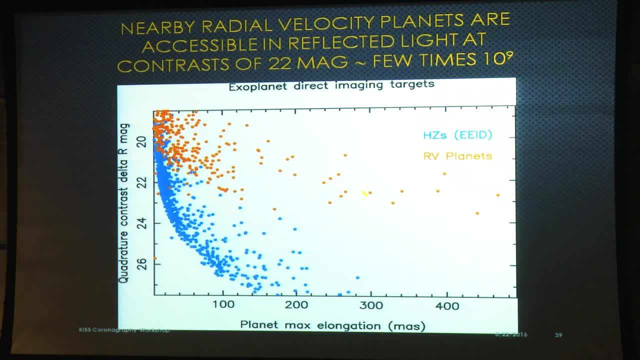 the 1 AU equivalent insulation distance. you can see that the known RV planets are at contrasts here that are becoming doable. This is around 10 to the 9 contrast here. This is about 10 to the 8th contrast there. 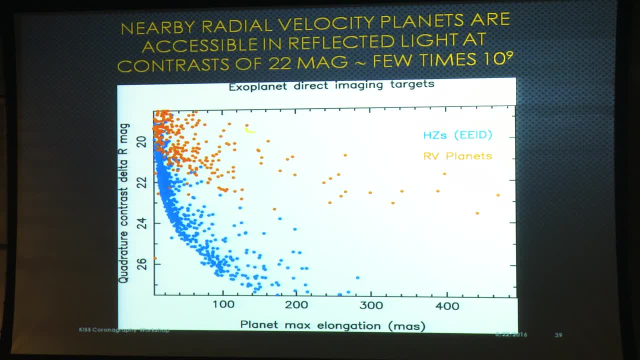 So this is a sample of nearby RV planets that WFIRST is hoping to get to. These are going to be too faint down here. This is a 10 to the 10 contrast at that level. All right, but 10 to the 10 is what you need. 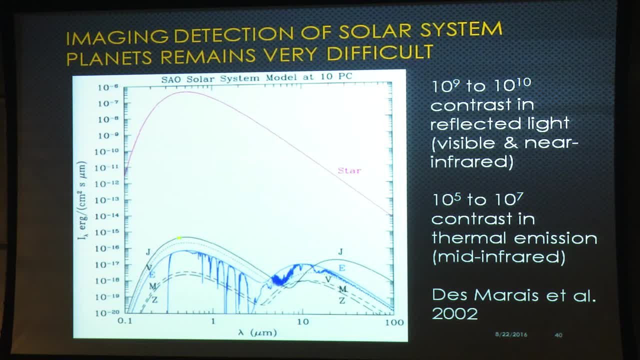 to go from the stellar signal and reflected light down to the Earth over here, or 10 to the 9 for a Jupiter In thermal emission. it gets a little easier, but that's not an option NASA's pursuing right now. So to go and image these reflected light planets. 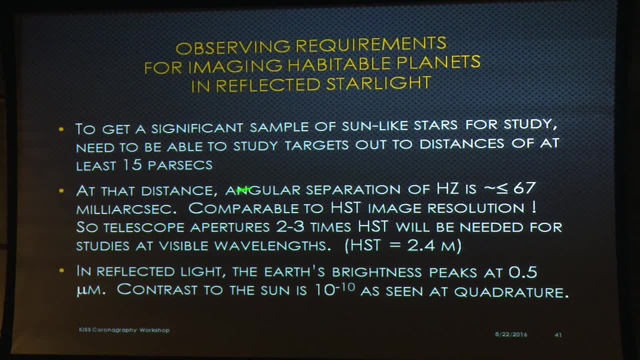 well, what do we need to do? Well, first of all, if we want to look for Earth, we need a significant sample of stars like the sun, where the contrast is 10 to the 10. So you're pretty much going to have to go out. 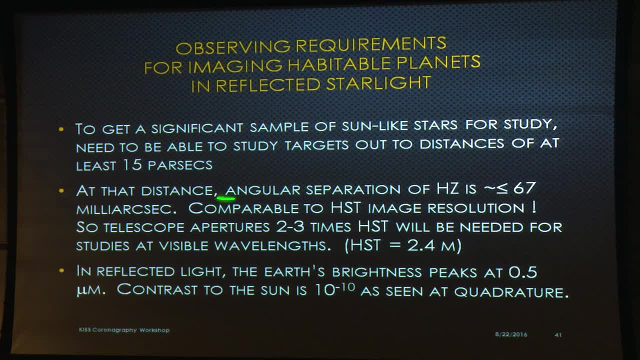 to at least 15 parsecs, and more is better, But of course when you do that, the habitable zone starts to expand. It's going to extend for a very short distance away from the star. It's getting comparable to the resolution of HST. 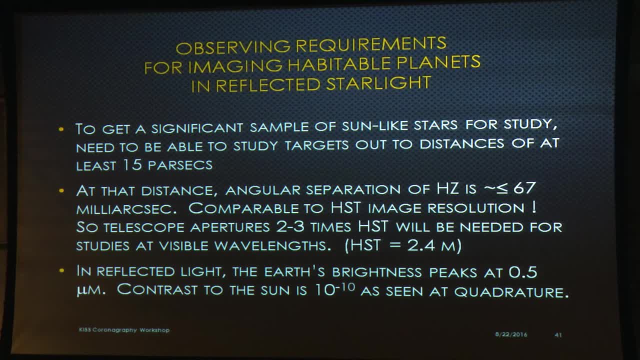 And you, basically for a coronagraph, can't look at one lambda over d with full contrast. You need to be at two or three lambda over d, so you're going to need a telescope that's two or three times the size of Hubble. 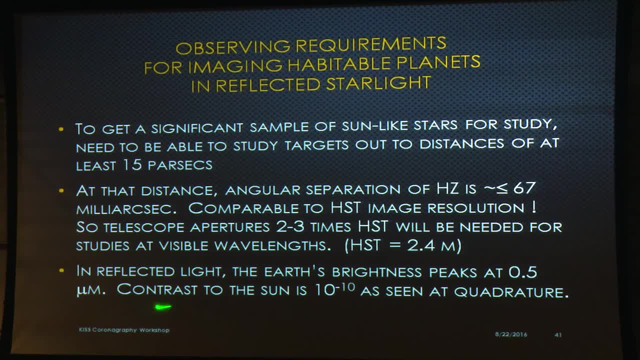 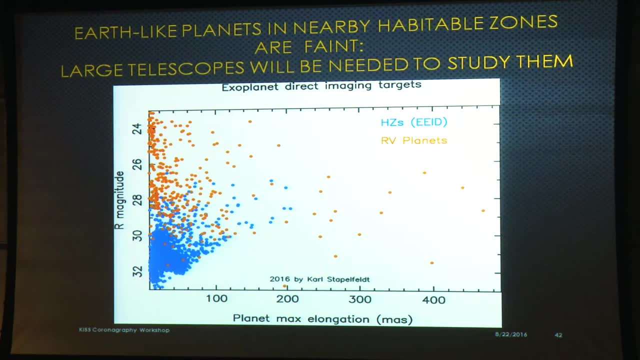 to do this at visible wavelengths, Then in reflected light, you want to do this at half a micron, where you have the best resolution and where the most signal from the planet. But the contrast, the absolute brightness, sorry- of the planets is still an issue. 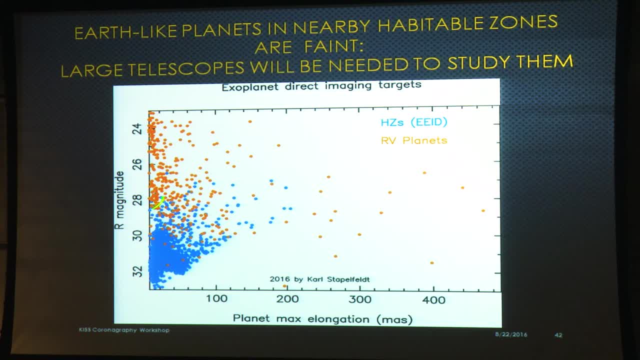 Here's the radial velocity planets now, not the delta magnitude, but just the absolute brightness at R band, And so you can see these are getting down to like 28th magnitude for the RV planets and the Earths don't really start coming in. 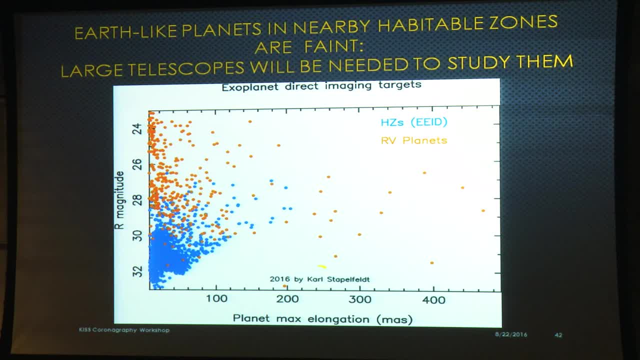 until you get to be 29th and 30th magnitude. So we don't have spectra from Hubble of anything that's 31st magnitude or 30th magnitude. It's just too hard and the efficiency of the system is too low. 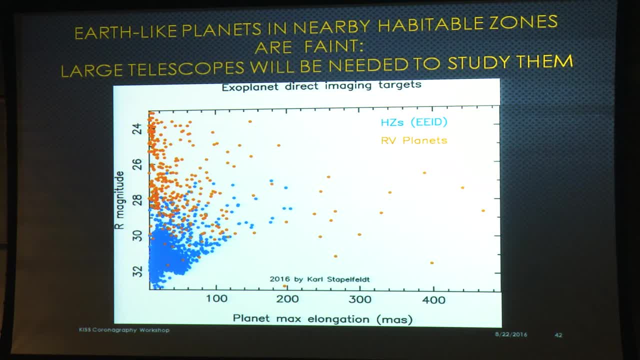 So it's quite a challenge to go and make a system that's going to be big enough, with high enough throughput to do spectroscopy at resolution of 70, which is what we think we need to detect the Earth oxygen analog signature. It's going to be really hard to do that. 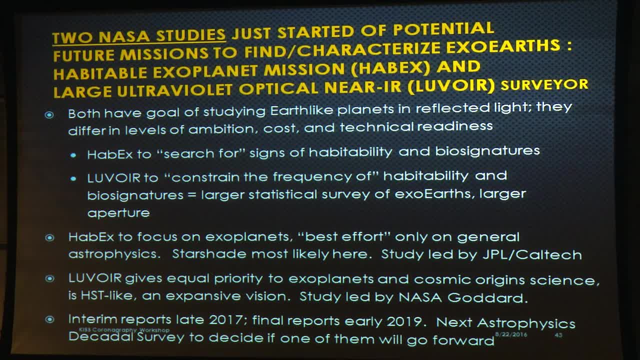 unless you go to quite a big telescope or look at a very small number of very bright targets. So we had an effort back in the beginning around 2000 and going forward that Chas worked on heavily of the terrestrial planet finder, first in the infrared. 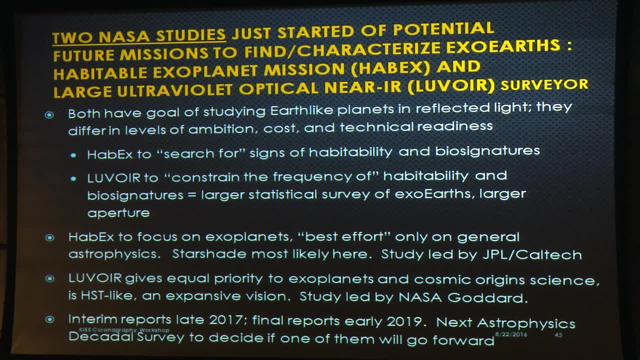 and then in the optical with the coronagraph. TPF was lost to history now. It wasn't able to go forward because the technology wasn't still ready and JWST needed all the money. But we're going to try on a low level now. 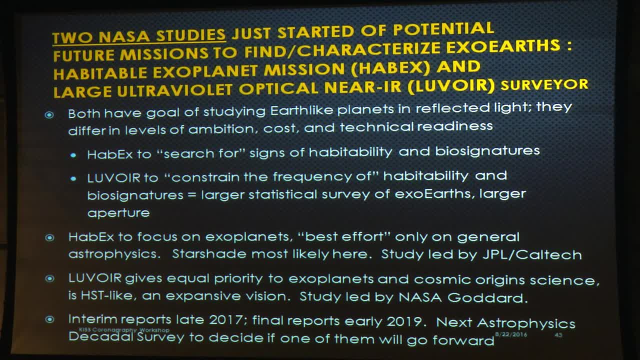 to get back to that direct imaging mission that we were thinking about 10 years ago, and that's the process of the upcoming decadal survey. NASA is doing two mission studies, one called LUVOIR, one called HABEX. I can describe them more fully. 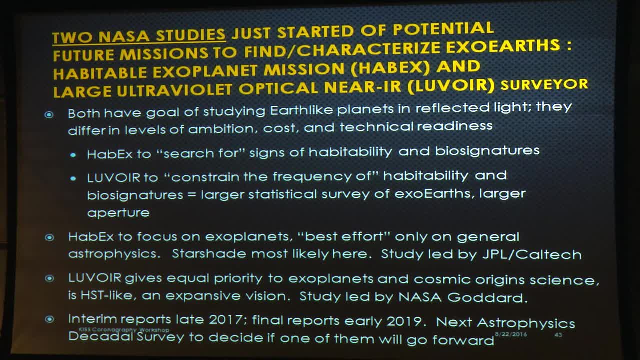 We'll talk about that afterwards in the discussion, if you like, And the idea is they would both have the goal of studying Earth, light planets and reflected light. The difference between them is just how ambitious they are and maybe how much they would cost in their technical readiness. 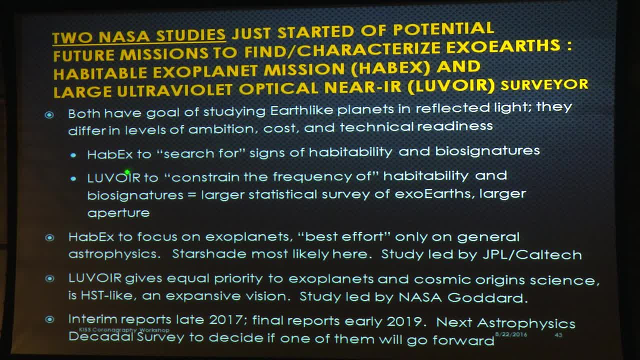 HABEX, the Habitable Exoplanet Mission- right now it's a study only- would be to search for signs of habitability and biosignatures. LUVOIR would want to look at a much larger sample and be able to get some statistical information. 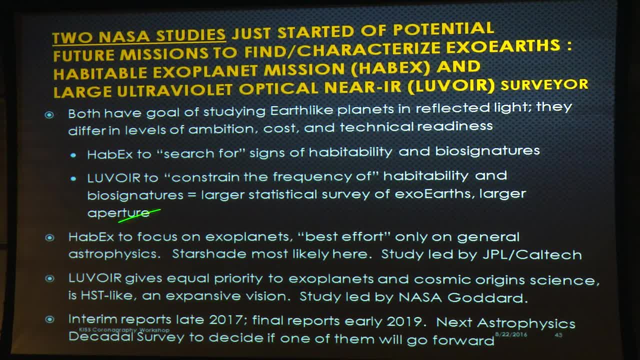 on the frequency of Earth analogs and different atmosphere types, And so the other difference that's important is LUVOIR is going to give equal priority to the Hubble kind of general astrophysics extragalactic, whereas HABEX will try to do some of that. 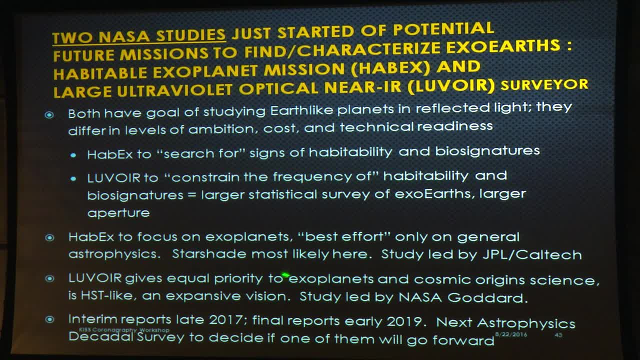 but only on a best effort basis. And these studies just started up at the earlier part of 2016, and by the time they get to 2019 they should be done and ready to tell the decadal survey what its options are, not only in terms of capability. 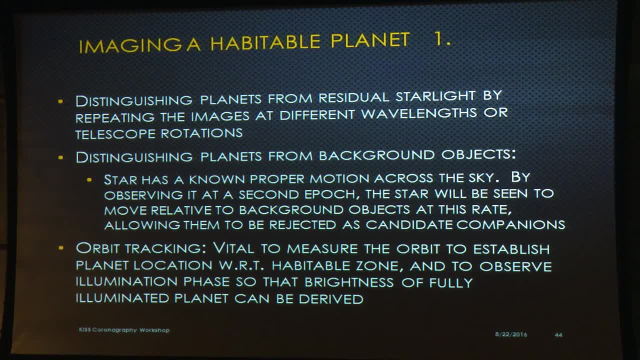 but hopefully in terms of cost. And so the kind of things that these missions have to do is they have to be able to distinguish planets from residual starlight, just as the ground AO observers are doing. You do that by observing at multiple wavelengths and making sure a speckle would change position. 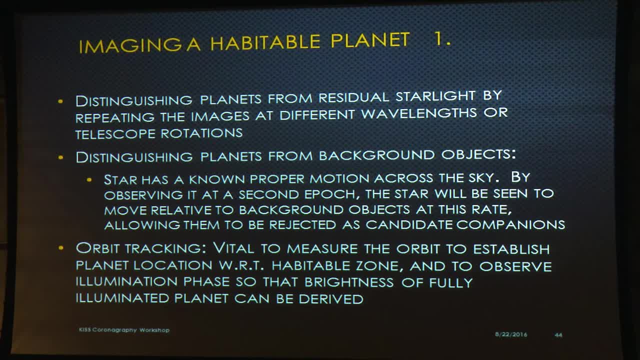 and a planet would not. or you rotate the telescope and see that the planet rotates with the sky, but the speckles don't rotate, they're fixed with a telescope. So we have these sort of techniques that will need to be applied so that the spacecraft have to have this capability. 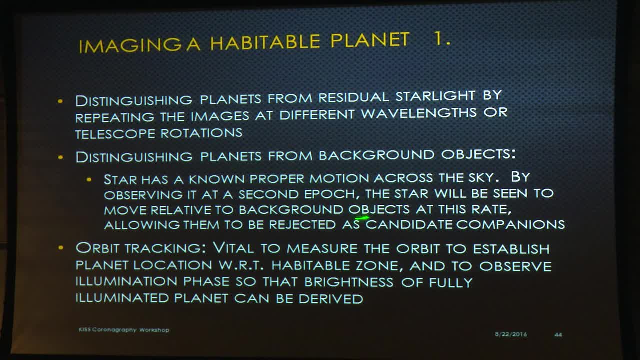 We have to be able to do proper motion observations to make sure that the object is a companion, and then go back and also measure at multiple epochs what the orbit is of something we would detect, so that the missions all have to build this into their baseline plan. 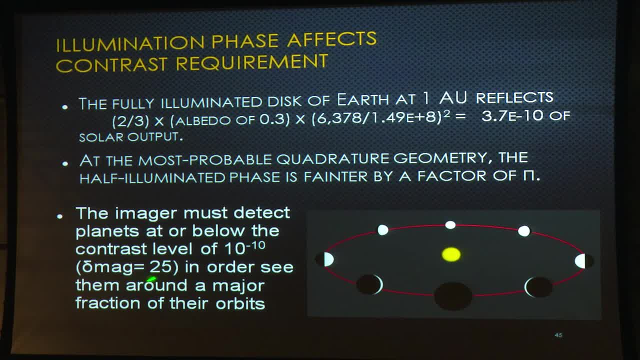 And then the contrast of 10 to the minus 10, 25 magnitudes is great for detecting the planet at elongation, but it might be seen partially in a crescent phase, If you want to be able to have some completeness in your observation. 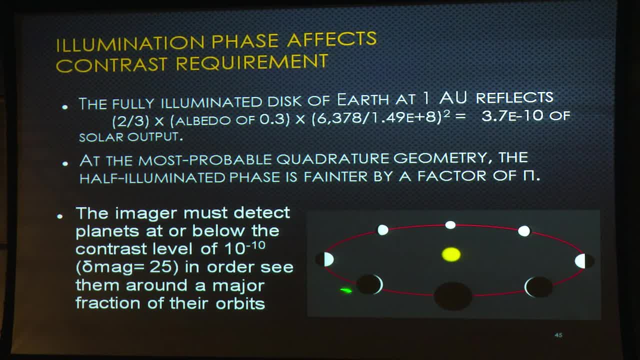 you need to be able to actually integrate deeper than that. if you want to see it somewhat towards the near side, And of course you might say, well, why don't I just observe it when it's fully illuminated, like over here? but the occulting spot of the coronagraph 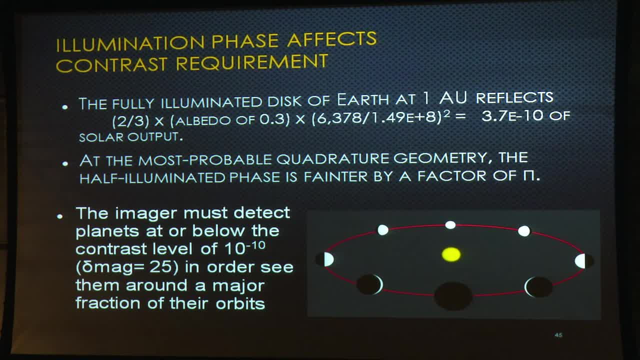 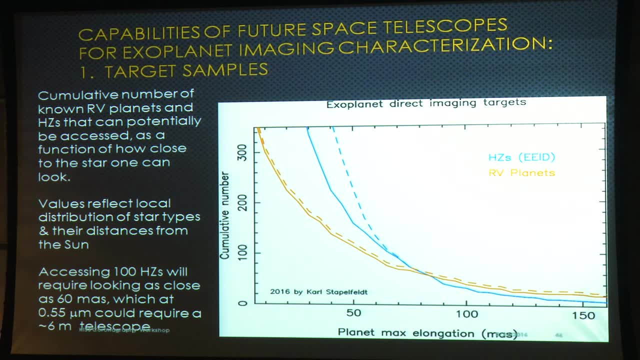 for many systems will be so large that you won't be able to see these gibbous phases, so you can't count on them being accessible in general. So then, the size of the telescope, the sample you can look at. go and look at the Hipparcos catalog. 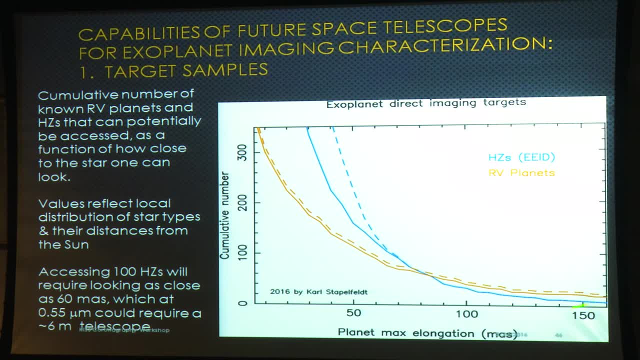 calculate your habitable zone sizes and then their angular sizes on the sky. do that the same for radial velocity. you get these two curves here. So let's say your telescope can look in to 100 milliarc seconds in a working angle. 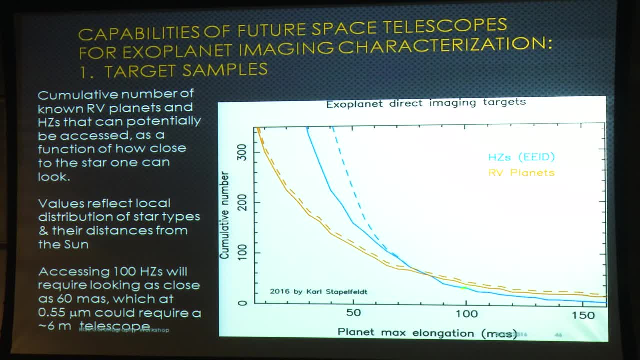 If that's the case, then you can only access about 15 habitable zones. oh sorry, that's 30, 30 habitable zones and then in terms of RV planets, you're getting maybe up to 40. But if you can go in closer to say 50,. 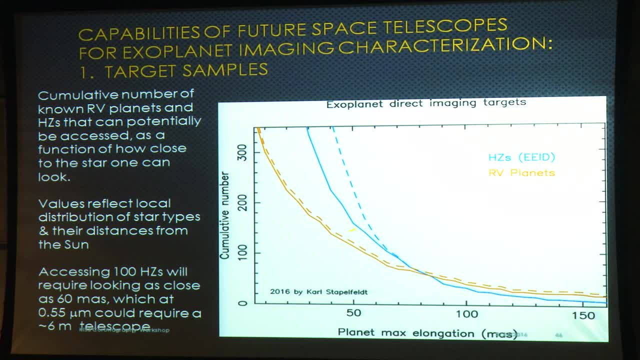 or you can go to 40, then now you're getting into something like 140 habitable zones and maybe 100 RV planets. So you win big if you can go in close, And then again, I hope that's one of the themes of the workshop here. 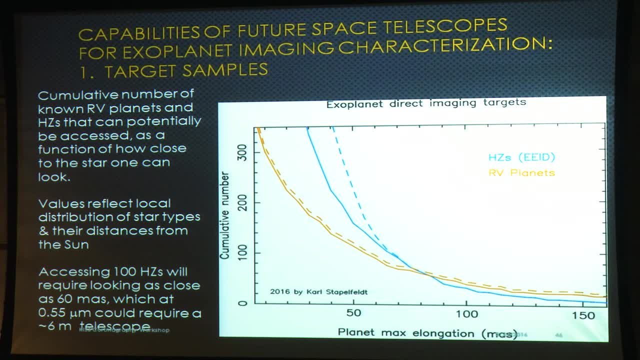 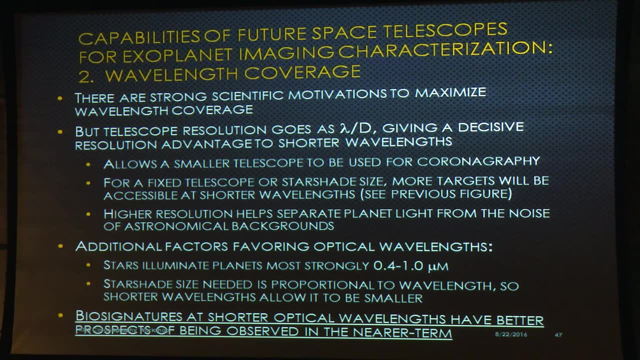 is: how do we do the best we can, going really close to the inner working angle? This is the motivation for it. So, then, another thing that we want to be able to do is look at multiple wavelengths. I won't go through all this. 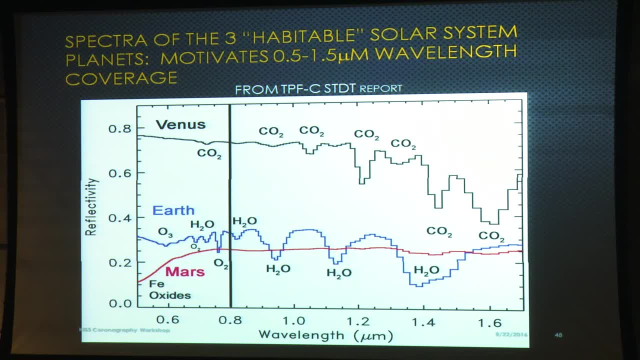 but I'll just show you the next slide from the 2002 Desmarais report showing the spectrum of the Earth across the optical and the near infrared and all the various features, especially the strong water features, that come in if you can go into the near infrared. 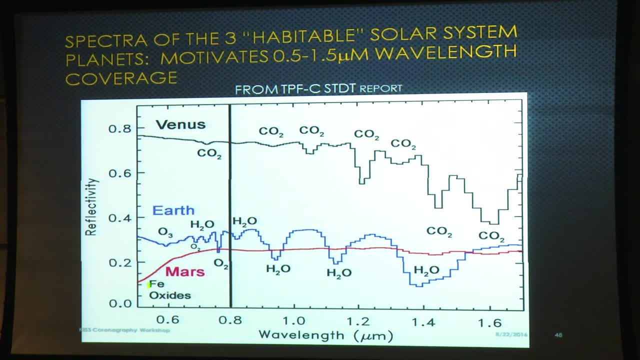 Venus has strong CO2 features. Mars, with hardly any atmosphere, doesn't have strong features, but you can see a little bit of the CO coming in there. So the main point of this is that both HABEX and LUVOIR need to consider a near infrared capability. 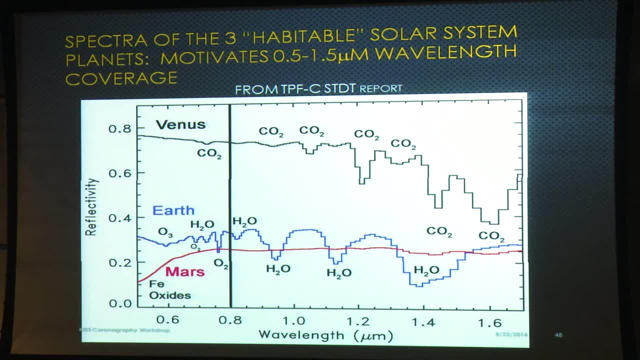 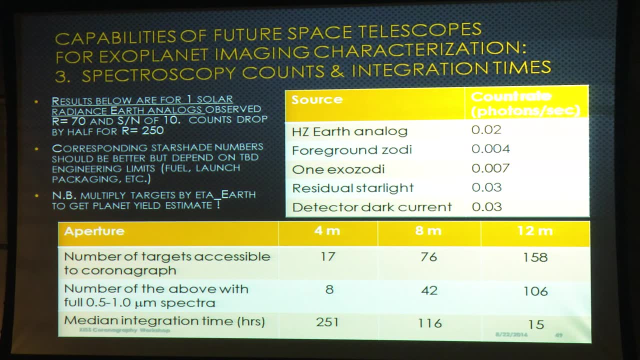 for as many targets as they might be able to access. Otherwise we're just not going to know, for example, if it's a large CO2 atmosphere. But I want to impress upon you that this is a hard problem. So let's say you take telescopes of different sizes, 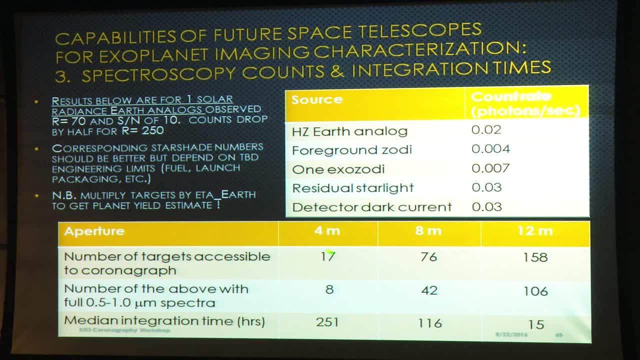 4,, 8, and 12 meters. It turns out for the number of targets you can access. here you have these signal levels and then if you get a bigger telescope you can access more targets, but the average signal level of those fainter targets 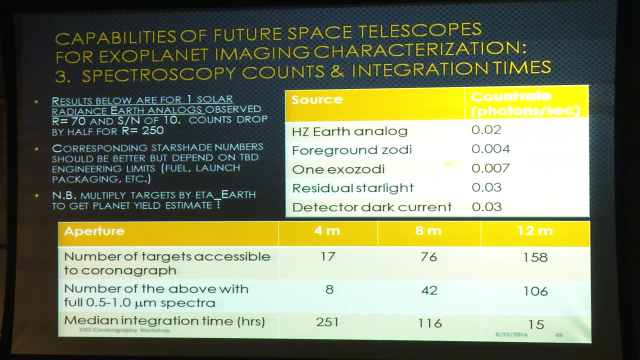 is still about the same. We're getting, even with these large apertures, you know, one photon a minute from an exo-Earth planet, And then they've got these other backgrounds around here, the sky background in the solar system. 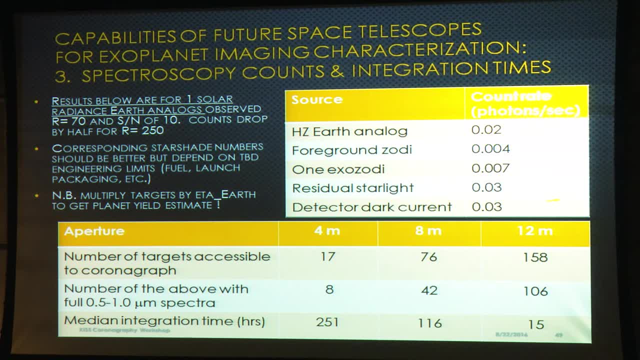 possible dust in the exoplanetary system, residual starlight. So all these things contribute to make the problem difficult, And the ZODI in the other system- the dust particles there and the scattered light they produce- is still not well constrained, And so that's the faint signals. 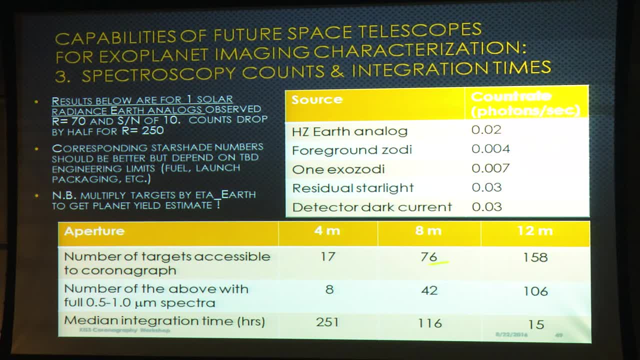 and this is just from inner working angle considerations, how many of these you can do. And even if you can access a planet, it doesn't mean you can see the spectrum over all the wavelengths. Typically, the inner working angle is getting bigger as you go to longer wavelengths. 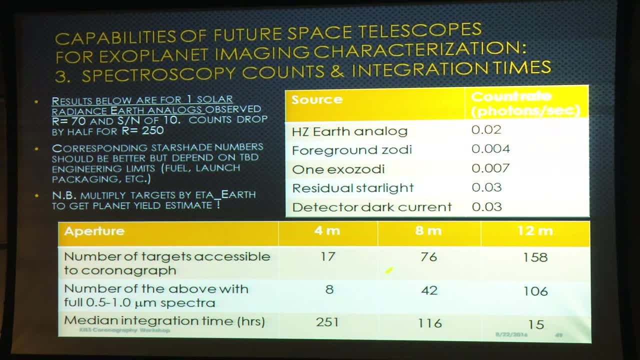 and so it's cutting off parts of the spectrum that you want to see. So an eight-meter telescope would access, you know, about 80 habitable zone targets, but only about half of them would have full spectral capability. You can see the integration times here too. 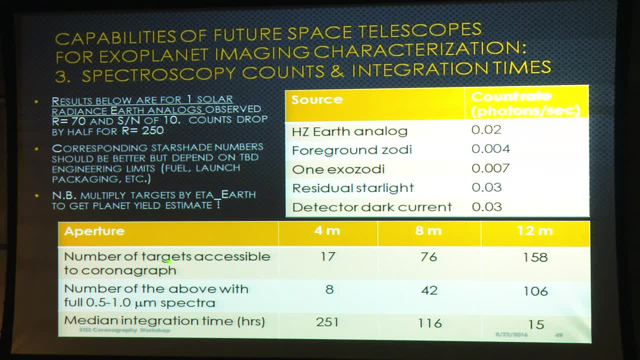 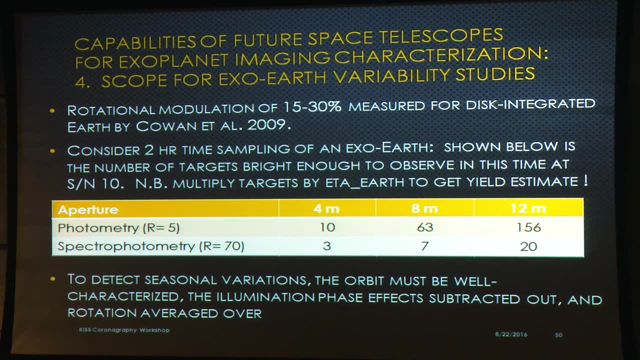 Multiply all these numbers by whatever you think Eta, sub Earth is to get the actual yield that the mission might have. And so one of the last things I'll mention, a capability we'd like to have for these future direct imaging missions- is to look at variability in the planet's signal. 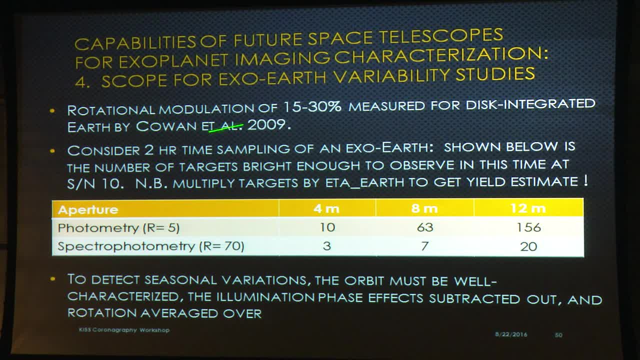 And in reflected light. this is something that was observed by the Epoxy mission back in 2009,. the repurposed Deep Impact spacecraft looking back at the Earth and watching it rotate The features on the surface of the Earth modulated the total integrated brightness. 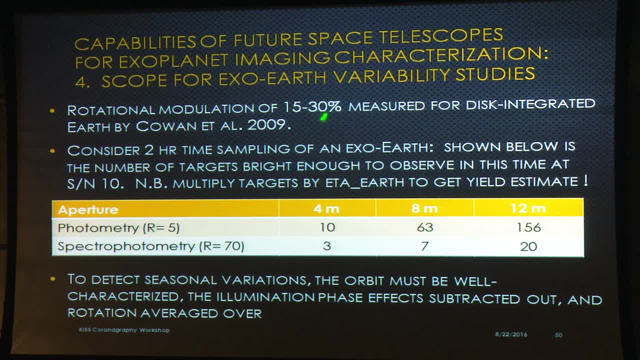 by about 20 or 30%. So if you want to be able to measure that sort of in two hours seeing, you know, continents rotate under view, for example, or oceans- then the number of targets where you can do that photometrically. 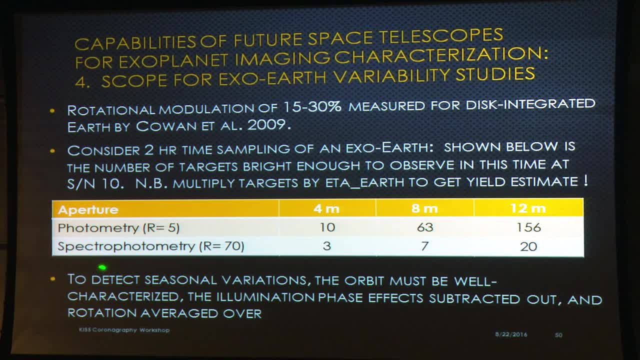 is shown here, Multiply by Eta, sub Earth, And then, if you want to take spectral photometry of these at the same time, it's even smaller. So, while these are great things to talk about, we've all loved the rotation rate of the planets in the other solar system. 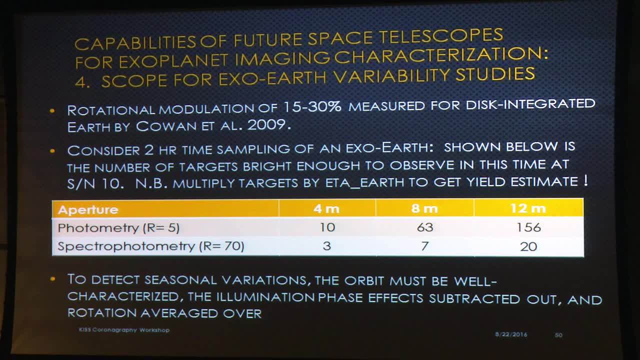 it's not going to be doable on a large fraction of their available targets. And you can talk about looking around the year as the planet orbits and seeing seasonal variations. you know the Martian ice caps become very prominent reflectors at some times of the year and other times of the year they're not. 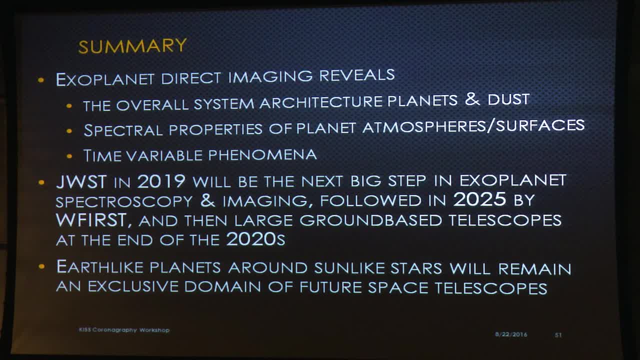 So that's something you might hope to see in an exoplanet. So, to wind up, imaging is going to tell us. unlike the other techniques, sort of in one quick, deep image, it could show us the planets that are there and the dust structures and their 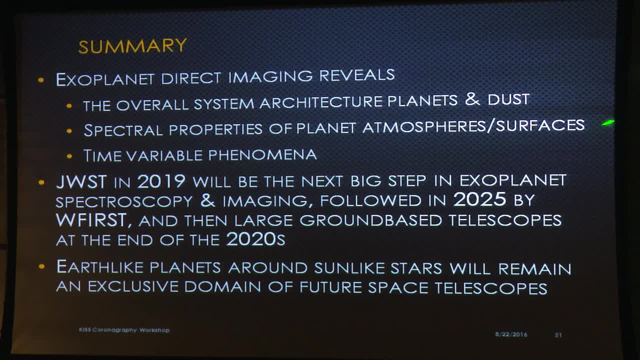 spatial relationship to each other. It tells us all these things about the atmospheric composition and if you have a very transparent atmosphere, maybe the surface is too And maybe the time variable phenomena I just mentioned. So JWST's major contribution coming up is going to be a transit spectroscopy. 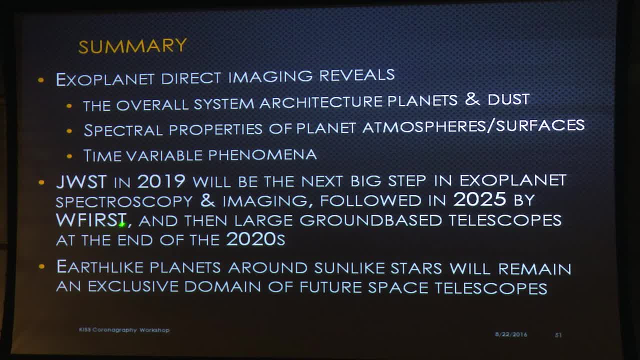 but there will be imaging Then WFIRST in 2025 on a small sample of known radio velocity planets, And the ground telescopes like TMT are hopefully going to get big instruments for adaptive optics and contribute at the end of the 2020s. 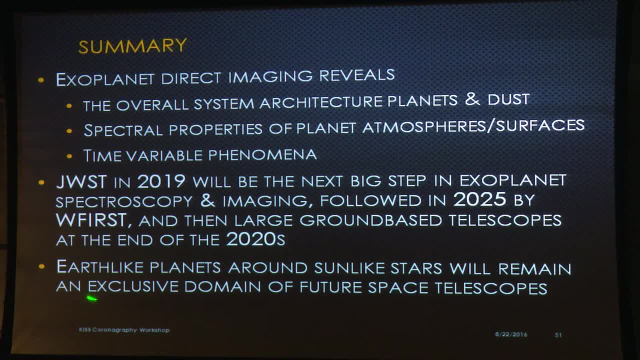 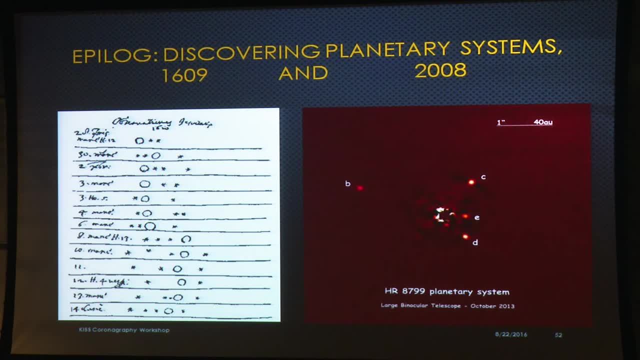 We hope to get to 10 to the minus 8 contrast from the ground, but 10 to the minus 10 still looks like it's the domain of space telescopes above the atmosphere, And the last thing I wanted to say is that over 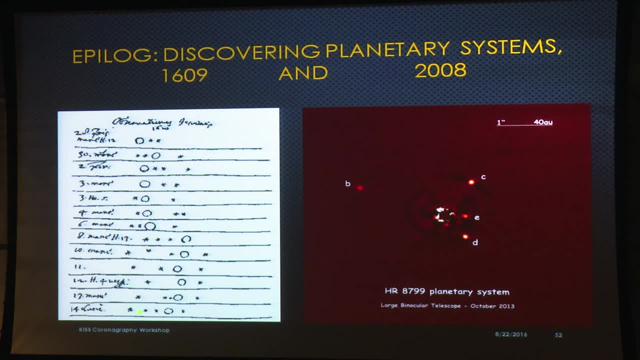 400 years we've gone from imaging a multiple planetary system, kind of Galileo with his little telescope, and see something that to me is very reminiscent: instead of the edge on kind of orbit of the Galilean moons, we've got the face on orbit of the HR 8799. 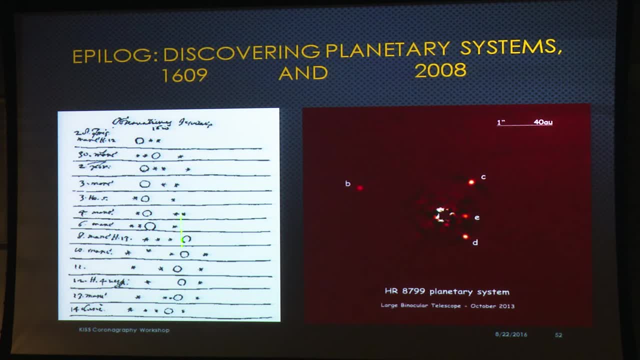 planets. But think about all that's happened in the 400 years since this observation was made. and think about all that can happen in the next 400 years since this observation was made. Maybe we'll go there, or maybe we'll just be making the biggest telescopes. 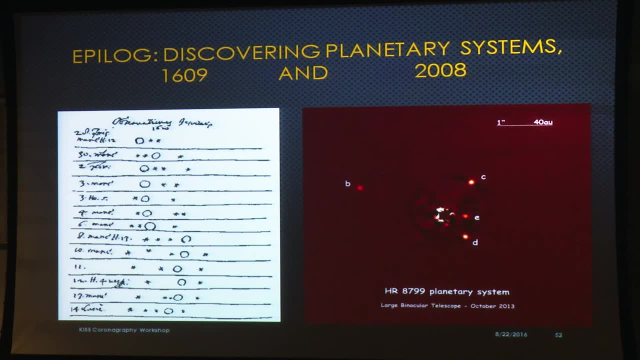 that we couldn't imagine now, And that's what I had to say. Thanks,